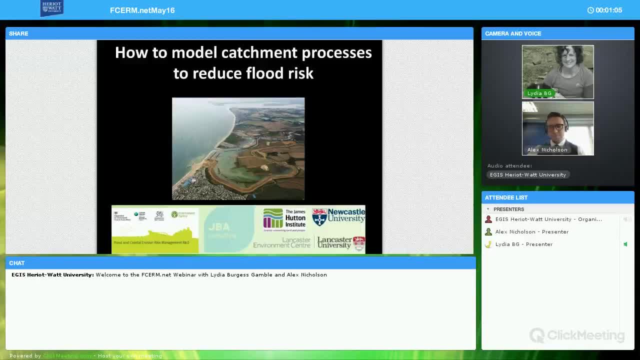 he's been managing and then hand over to Alex. So over the last year I've been managing a project with JBA Consulting to look at how to model catchment processes as part of flood risk management planning. Your project has been managed by Barry Hankins from JBA with subcontractors from the James Sutton Institute. 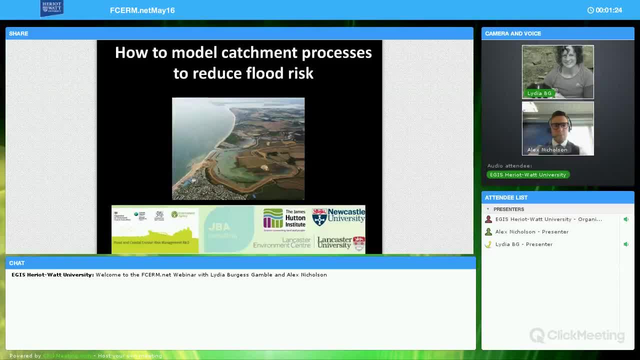 Newcastle University, Lancaster Environment Center and Lancaster University And it's a project that's been managed for seven years. I've been managing the project for seven years. Environment Agency and DEFRA Flood Risk Management Research Programme and we're basically a research programme that undertakes flood risk management. 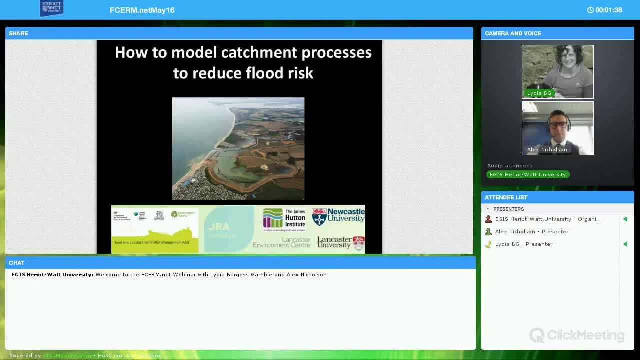 research for all flood risk management authorities in England and in Wales. For this particular project, we also had quite a lot of input from the SEPA, so it's applicable to the whole country. So before I get started and tell you about the project, I'll just give a little bit of context behind why we undertook this. 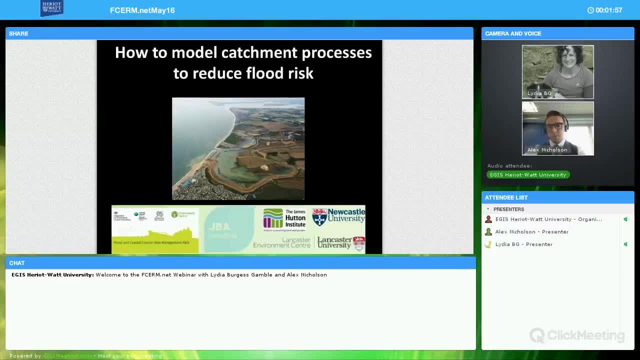 project. Over the last few years, as you'll all be really aware, there's been a lot of flood risk issues across the whole of the UK, an awful lot of flooding from all sorts of different sources and an ever-growing interest from a range of 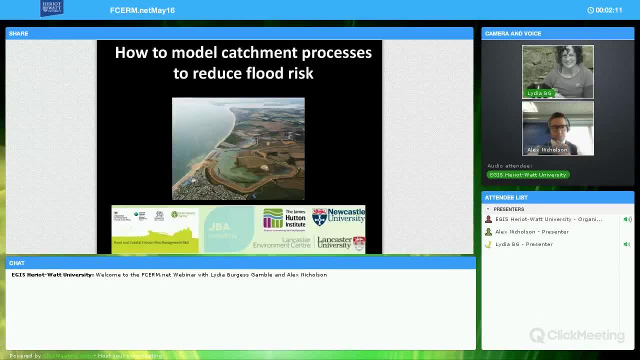 parties to look at a whole suite of different solutions to flood risk management, So to start to consider a wider range of solutions alongside traditional forms of engineering and, as part of that, call to look at a whole multitude of different solutions. there's been an increased interest in working with natural processes as a form. 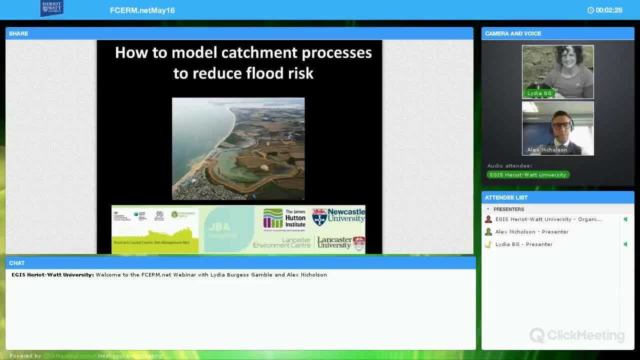 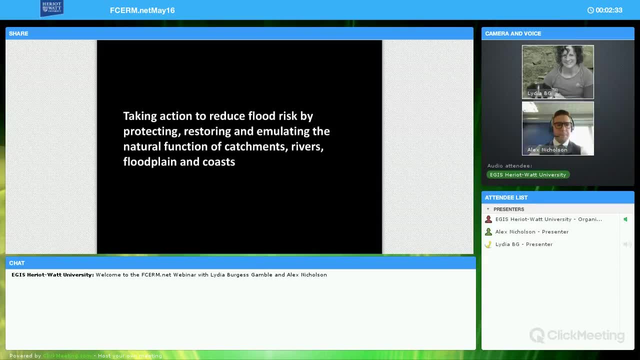 of flood risk management. Now, this form of flood risk management isn't anything new. Back in 2007, we were faced particularly in the 7 estuary and throughout many parts of the country. there was a review undertaken by Sir Michael Pitts into how the 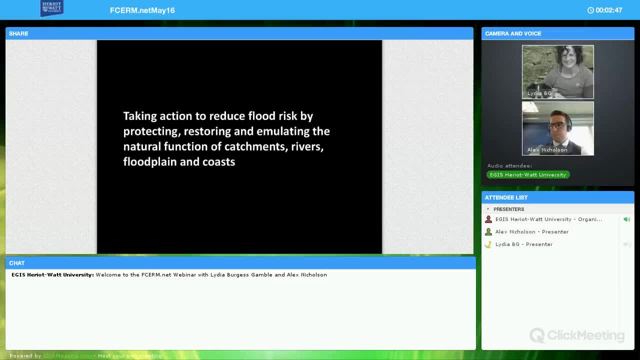 flood events happened and what could have been done to better manage those floods in the future. And as part of Michael Pitts review, he talked about how flood risk management should be a portfolio of different types of measures and should look at all sorts of different measures across catchments. 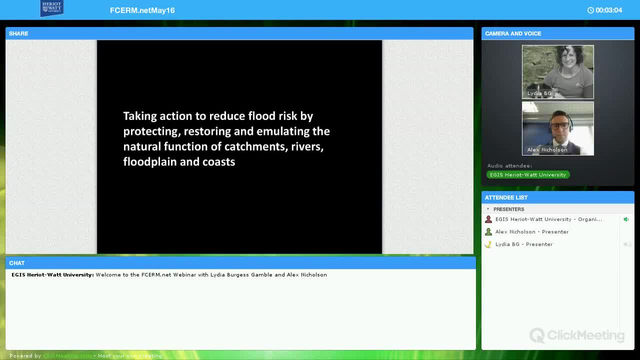 across coasts, in the rural and in urban environments to reduce flood risk, And he coined the term working of natural processes as a form of flood risk management. and he said that this is a form of flood risk management that's all about taking action to reduce flood risk by protecting the environment and by 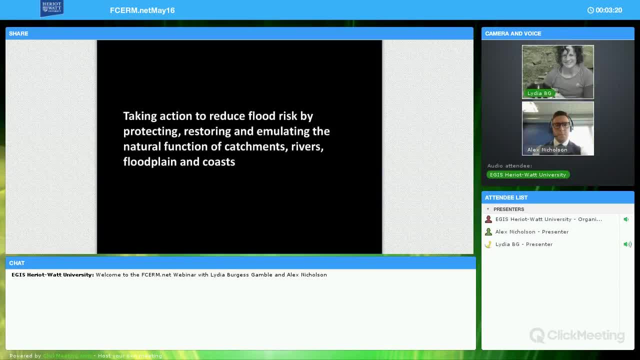 protecting, restoring and emulating the natural functions of catchments, rivers, flood plains and coasts, And it's not an approach that will work everywhere, but it's a really valid approach that we should be considering when we're looking at a catchment or part of the coast and asking ourselves what are the best. 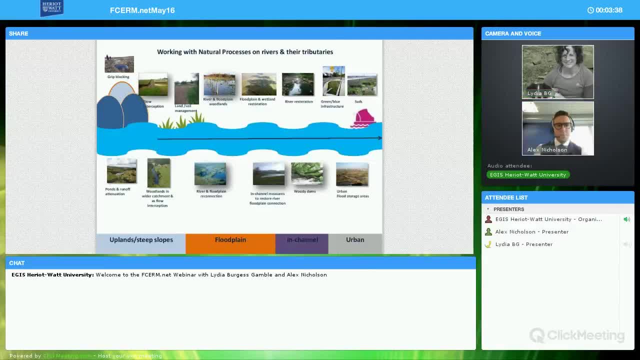 solutions for those communities who are at risk of flooding. Natural flood management, or working with natural processes, is a whole suite of different types of measures that are applicable on the coast and on rivers, and there's a wide spectrum of different sorts of measures that you might want to draw on from. 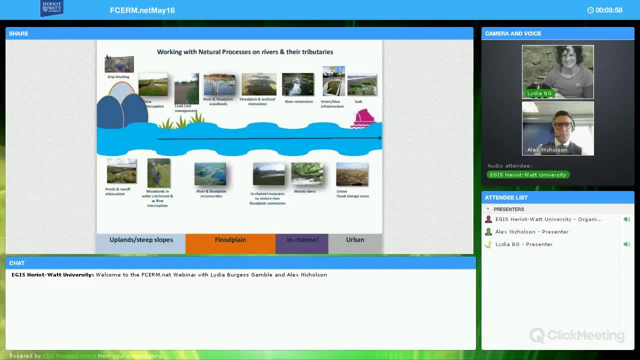 upland type of measures like grip blocking and intercepting flow paths to store water before it gets in the flood plain. through to planting woodland in wider catchments and in flood plain areas, through to flood plain restoration and wetland creation, river restoration and in the 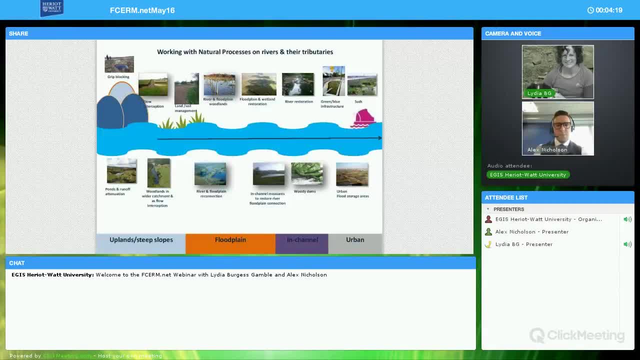 urban environments, looking at naturalised flood storage areas, green blue infrastructure and sustainable urban drainage systems. So it's a vast suite of measures and the types of measure you choose will really depend on your catchment type, on your geology, on the willingness of landowners and on the 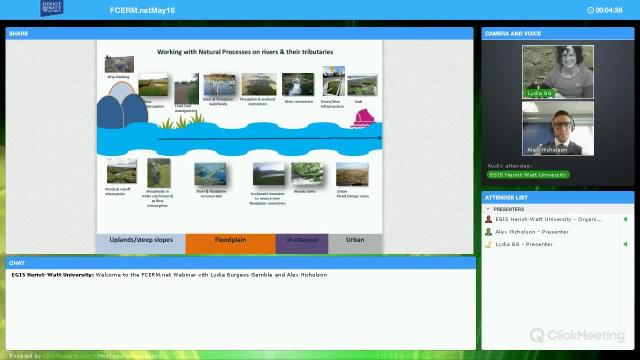 type of flood risks that you're trying to manage. There's a similar kind of spectrum of different sorts of measures and that you could see on the coast, such as managed realignment, restoring sand dunes to protect the coast from coastal erosion and each recharge, and 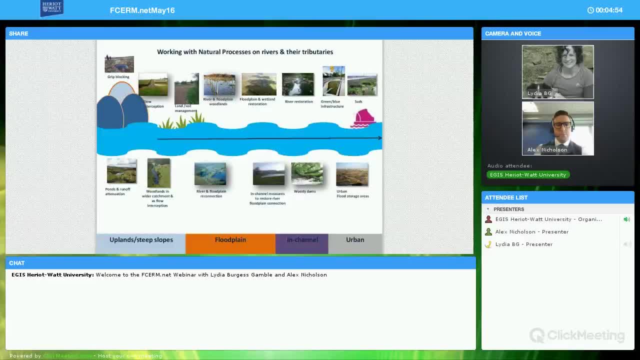 sediment management measures. So there's a vast range of different approaches, but what has never been done before is a review of the sorts of modelling that you might want to undertake and the sorts of data you might want to use to try and figure out what would be the best solution within your patch. So the real purpose of 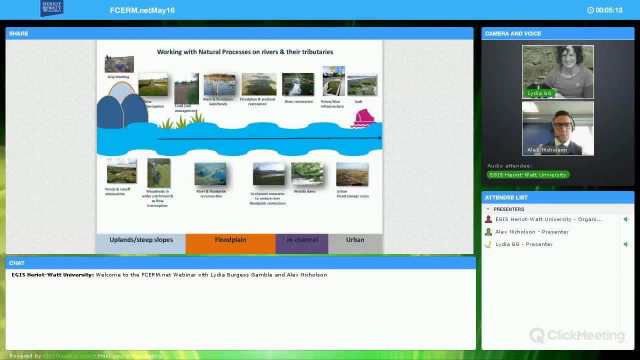 this project that JBA managed for us was to review what modelling had been undertaken for natural flood management schemes in the past and to get a bit of a flavour as to what the pros and cons of those different models are, and to develop a suite of products that can help you to figure out what you might. 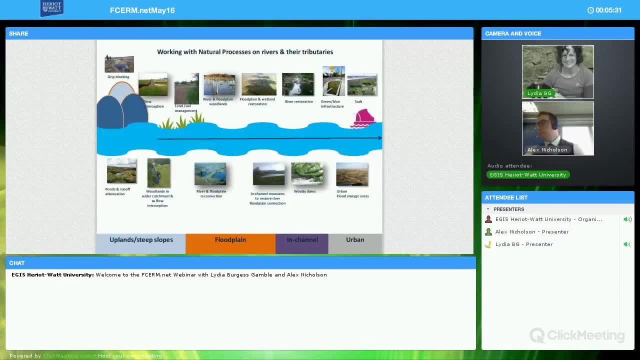 want to use when you're trying to develop a proposal for your catchment Indeed in some places. what we found was that you might not even want to do modelling. there will be cases where actually local knowledge and data within in that catchment can help you come to a decision without having to do modeling. 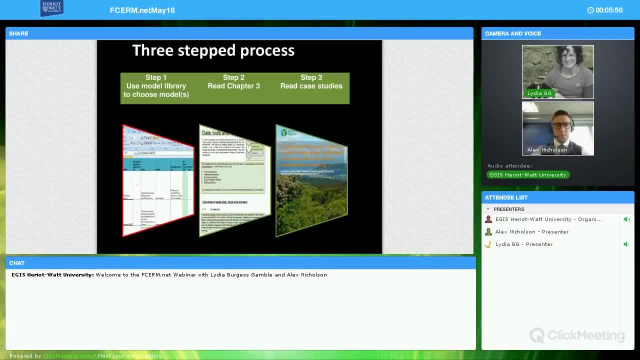 so the report, what JVA have done for us is they've developed a three-step process which helps you decide what type of approach you might want to take. they the reports and products that have come out of this study. we will provide you with a link following this, this webinar, so you can access those. they are all. 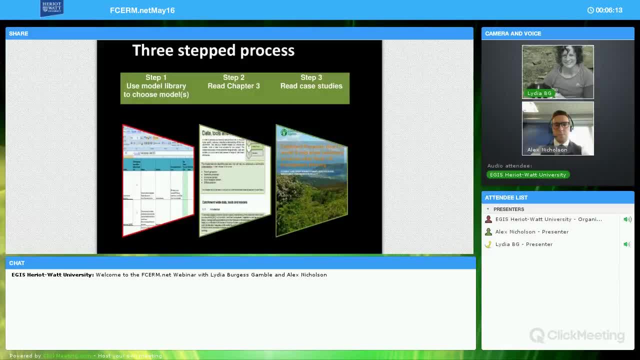 freely available on our Environment Agency Research page. but all I'm going to do now, before and before we go through to Alex, is to take you through the three different steps that fall within this JBA report, and hopefully you'll find that some of the products will be useful to you and your day jobs. 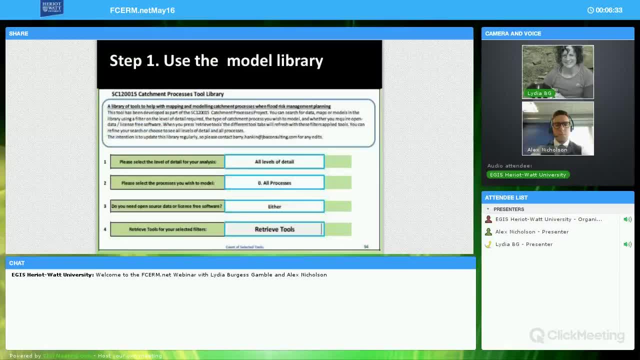 so the first step in selecting a model for your catchment is to have a look at our model library that we've developed. this is an Excel spreadsheet with three different models that we've developed, so we are going to go through the three different models that we've developed. this is an Excel spreadsheet. 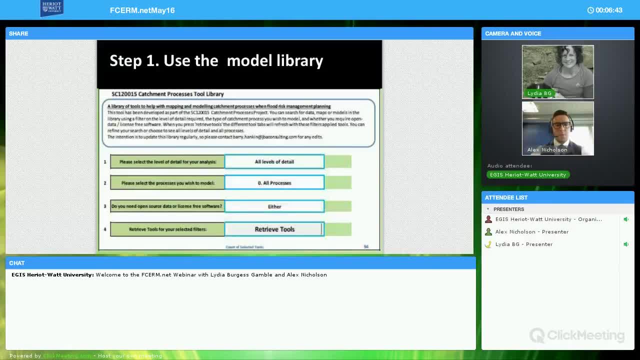 several hundred models, data and tools within it, and it has a front end that enables you to filter based on information to do with your catchment, so you can go into various different levels of detail, depending upon the types of natural process that you're trying to model, whether you want open source data. 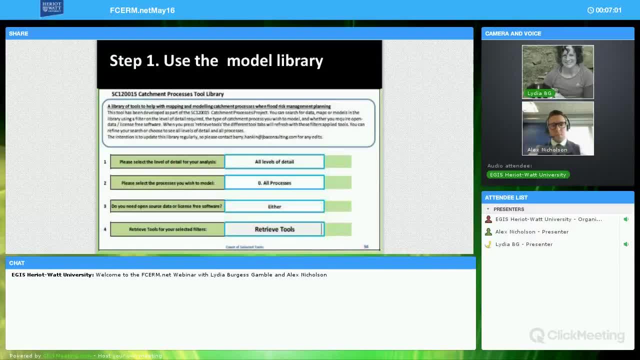 or whether you don't mind getting obtaining models that need software license, and and by clicking on on these boxes, it filters all of those models that are within the spreadsheet and puts forward ones that might be appropriate for you. what we had hoped was that there would be, with uncover, some magic model. 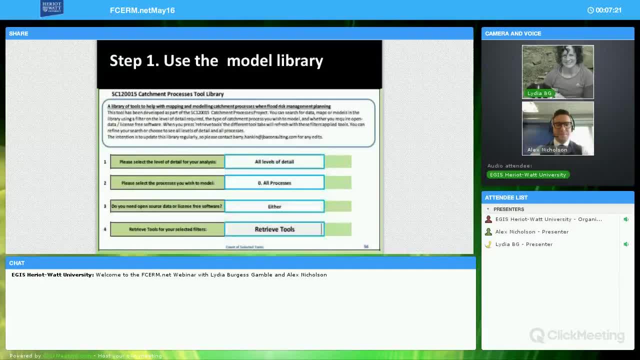 that would be amazing everywhere and that it could look at all sorts of different catchment processes. but what we found through this study is that there's no one singing or singing or dancing model that will suit everyone. it's really quite. it's really quite specific to your catchment, your geology within your catchment, what local 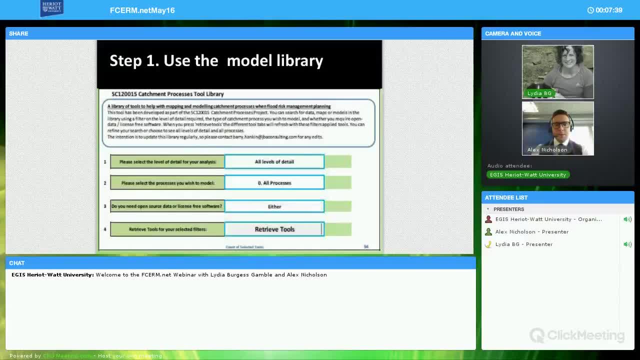 knowledge. you've already got around models, what models already exist within your locality and often, often, that is perhaps sometimes a more important process than trying to find what model that suits every, every situation. so knowing what models you have at your disposal within your organization or within your local environment agency team is also a really good process. so 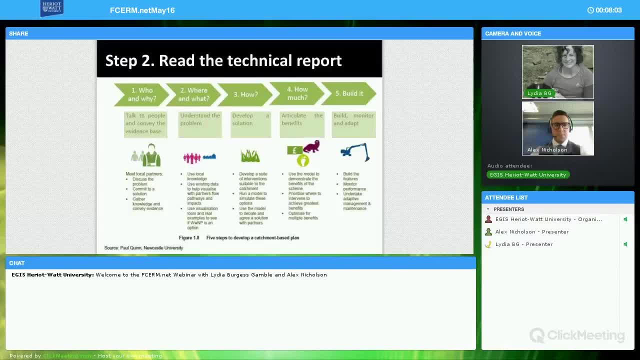 the model library is really helpful, but alongside the model library we have a really useful technical report which gives some general information on the steps you might want to go to, from thinking about a potential way of reducing flood risk to actually getting down on the ground and building it. so there's steps within. 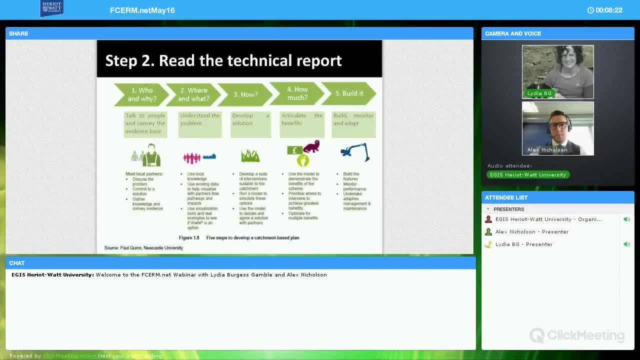 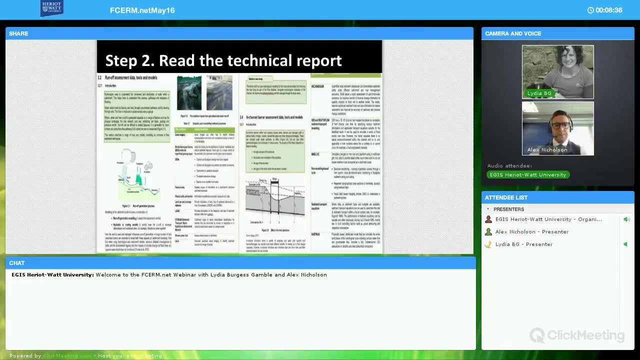 this report that help you think through at what stage would you need to think about modeling and how you would figure out which data and models are available to you. within that technical report there's specific chapters on different types of catchment processes and it describes in detail the range of different sorts of 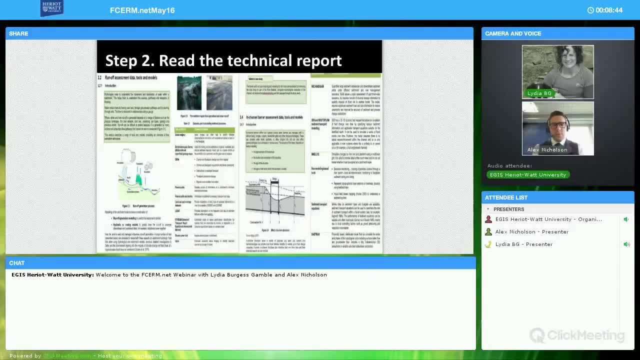 data and tools that are out there and what the pros and cons of those are, and will give you a really useful insight through the use of case study vignettes to understand where where these approaches have been used in the past. what's really good part of the report is that a company's 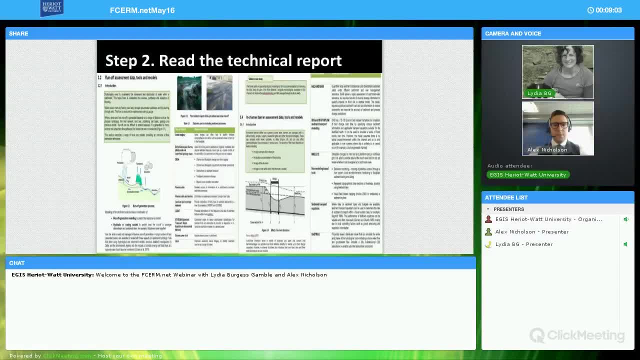 thinking about what can they do to address this challenge. so just to give you a little bit of background, what a lot of what we've been trying to do in the case study is. we've been working on a lot of studies and, as i said in the 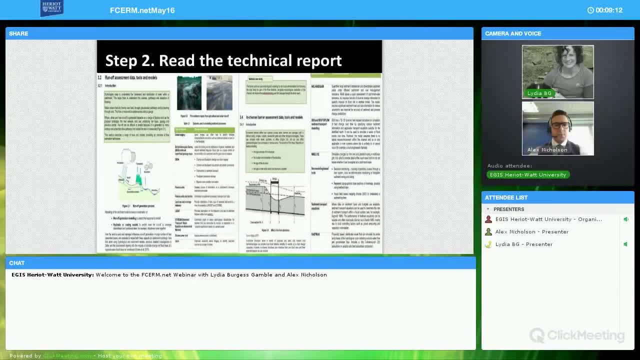 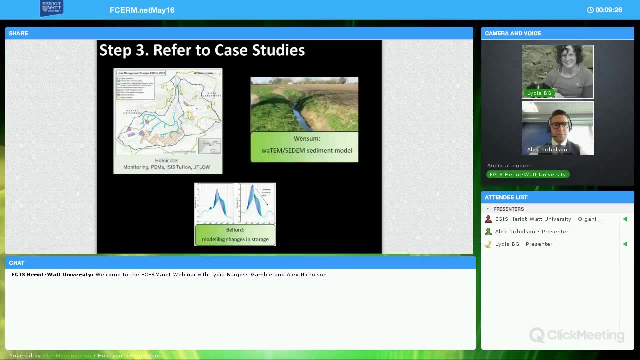 beginning the report are 20 different case studies from across the UK and these case studies are specifically designed to look at how flood risk and sediment management was modeled. within specific case studies. they cover a wide range of different types of catchment from all over the country and I'm just going to take you through a few now before I hand over to Alex, whose one of the case studies has related to the project he's been working on. so some of these actuals are based on data, and what does that mean. There are several types of data that are based on data, and what does that mean. 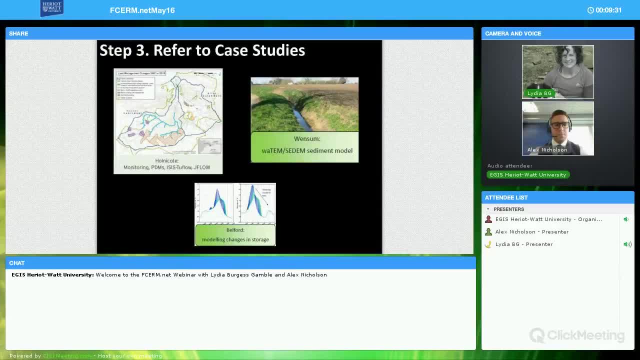 we've got a range of different examples. We've got some of the more familiar case studies, such as Belford and Holycock, which are quite well-known natural flood management schemes and some quite detailed case studies for those. We've got an example of some sediment modelling that was undertaken on the 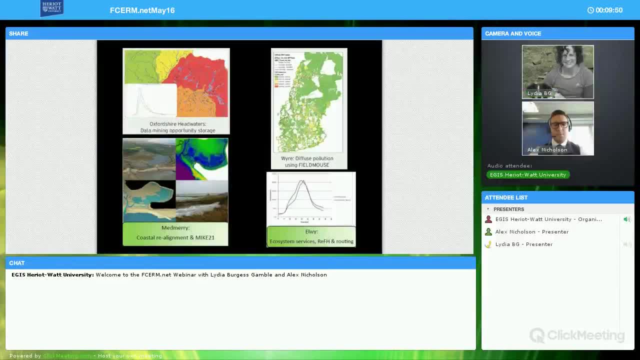 Wensum, on the east coast of the country. We've also got one coastal example in Medmurray. You should say this report was predominantly focused on fluvial situations, but we were given a really useful case study that we thought we would showcase nonetheless. So we've got Medmurray, we've got an. 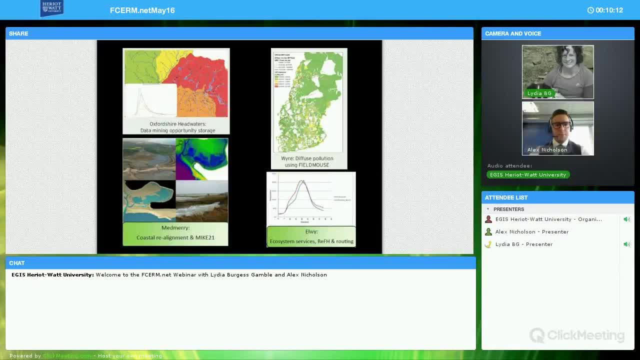 example in Oxfordshire on the headwaters where the NFU are doing some work to try and identify natural flood management opportunities. We've got an excellent example from Wales on the Elwe where Natural Resource Wales have done some work to look at different eco-systems. So we've got an excellent example from Wales on the Elwe where Natural Resource Wales have done some work to look at different eco-systems. So we've got an excellent example from Wales on the Elwe where Natural Resource Wales have done some work to look at different eco-systems. 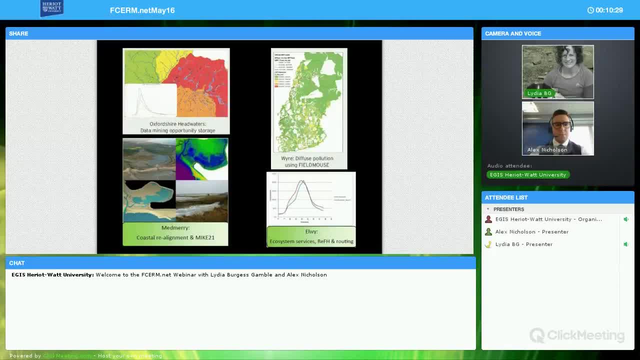 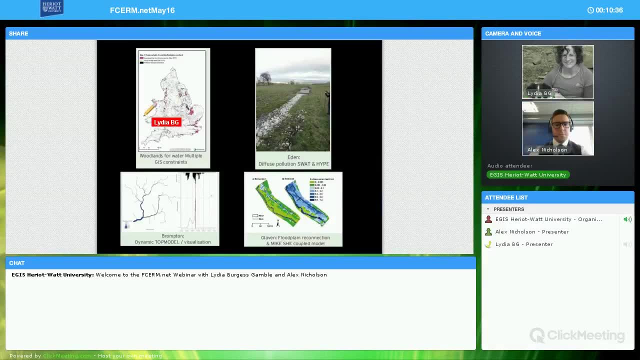 service functions within a catchment and where the best places could be for natural flood management. We've also got some examples of diffusion pollution modelling: A specific case study looking at the woodland for water opportunity, mapping, river restoration and diffuse pollution work on the Glaven and the. 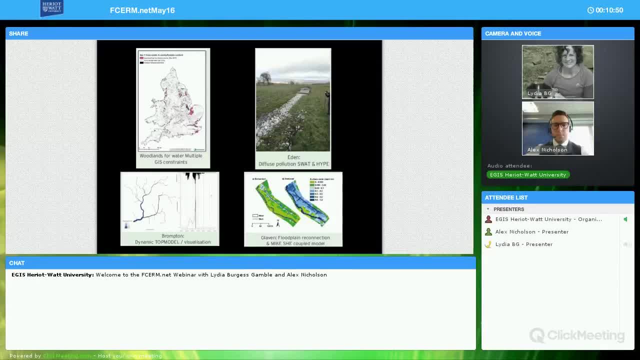 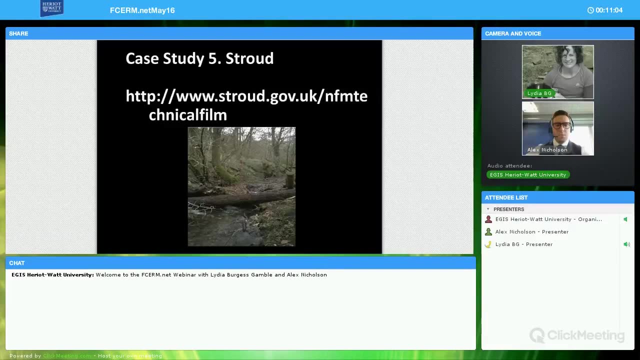 Eden And just click on to the next page and they're all really useful details, case studies that are definitely worth looking at if you think they might be appropriate to you. One of our case studies is the Stroud Natural Flood Management Scheme, which is a piece of work being led by Stroud District Council with 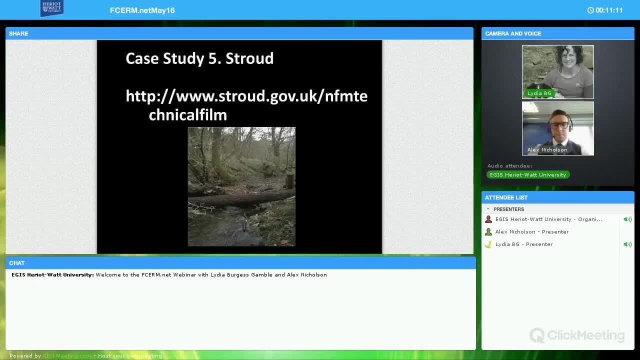 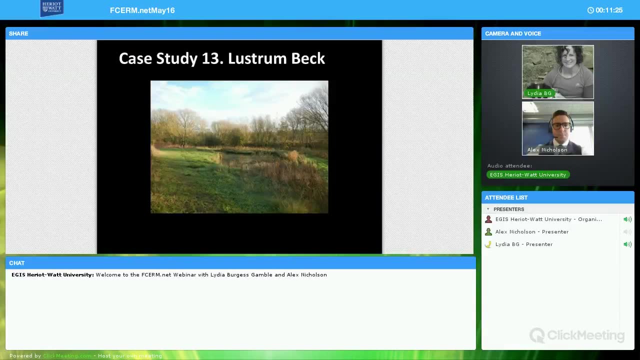 the Environment Agency and they've literally this week just published a really useful film that takes you through the practicalities of the work that they undertook within their patch, which is definitely worth a watch outside of this telecom. But one of the really excellent case studies we've got in our report is a project that Alex is working on at the 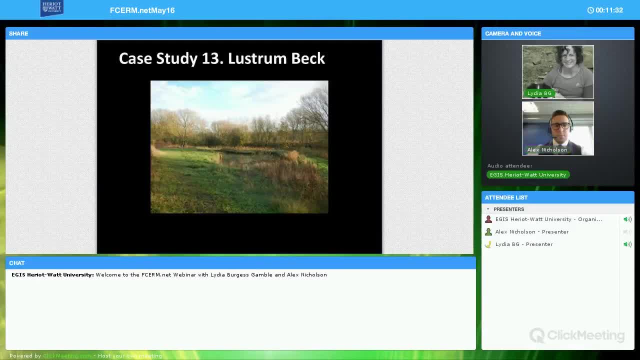 moment, and this is the case of the Lustrum Beck, which is in Stockton-on-Tees. So what I thought I'd do now is, in order to bring this report to life, is to hand over to Alex, who can take you through this case study in more detail, and 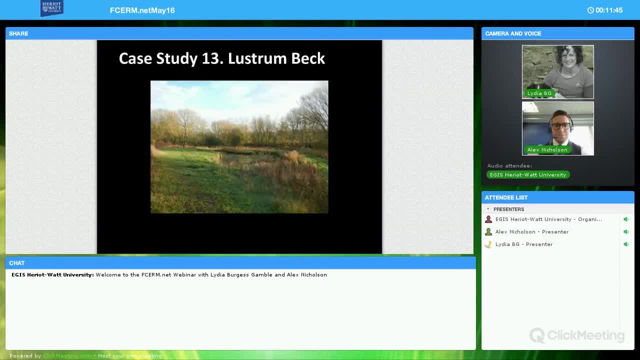 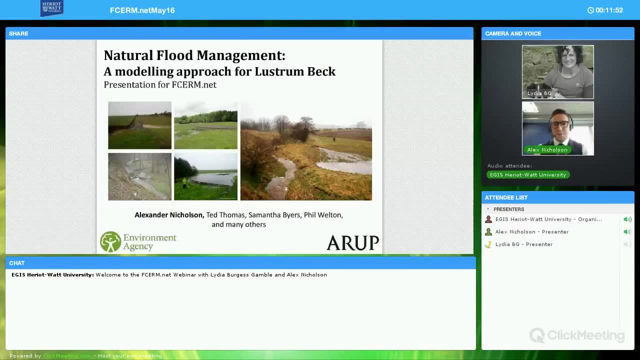 explain what he's been up to. So over to you, Alex. Thanks very much, Lydia. Yeah, so I'm Alex Nicholson. I'm a civil engineer and hydrologist at Arup, Currently submitted to the Environment Agency as an advisor to Natural Flood. 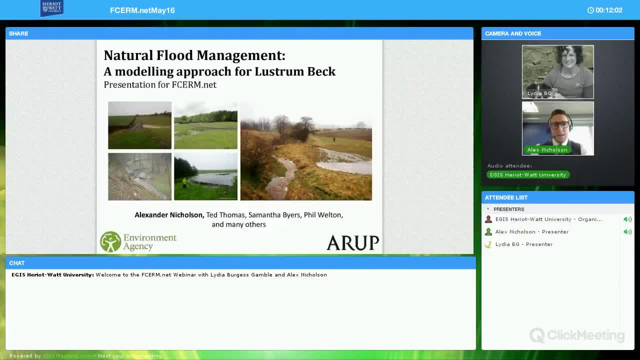 Risk Management. The photos on this slide are from Belford in Northumberland, which has already been introduced as an example case study. I just put them on there to highlight that some of the some of the research that I'll be going through has developed from from my PhD research that I undertook in. 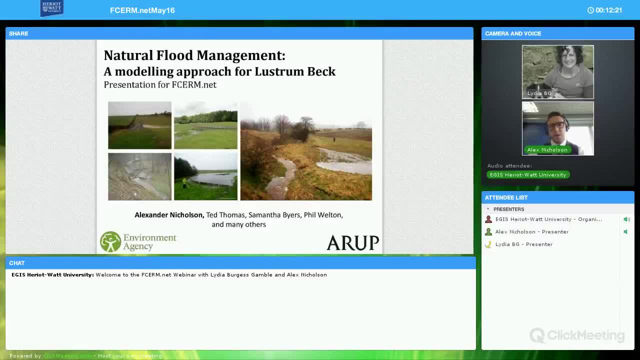 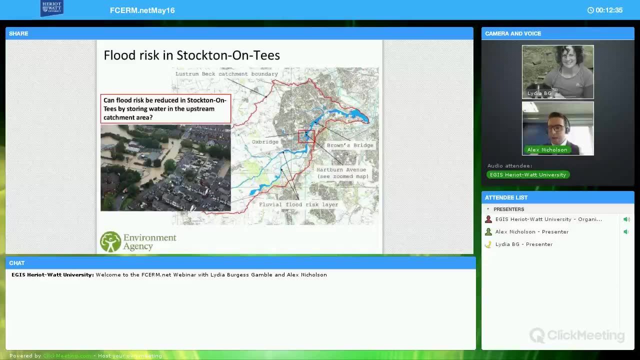 Belford. As Lydia's already said, I'll be talking to you today about the scheme in Lustrum Beck, which is upstream of Stockton-on-Tees, and we'll go on to that now if the slide changes. Here we go. So Stockton-on-Tees is situated downstream of a 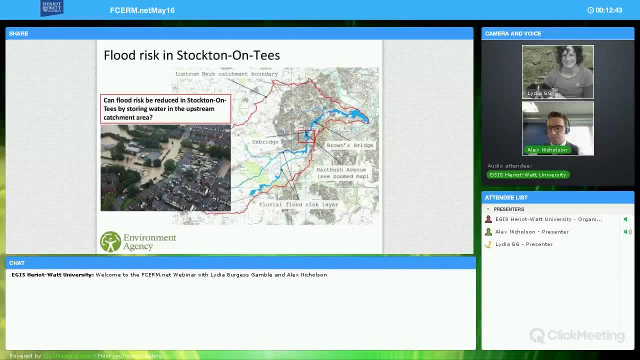 45 square kilometre predominantly rural catchment. It's a 3 million fence scheme is currently underway, being delivered in two phases by the Environment Agency in partnership with Stockton Borough Council. Phase one of the scheme is hard engineering: embankments, flood walls, bridge widening, culvert repairs and so 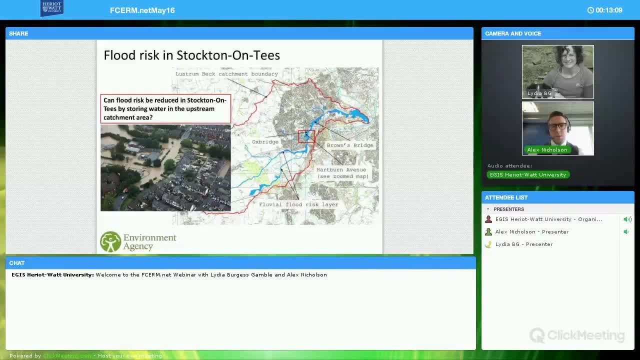 on, and these works are aimed to deliver protection to over 150 properties. Some of those properties further downstream into in the heart of the town are having a standard of protection raised to 1 in 75 year, and some of the properties closer to the upstream end of the town are only able to achieve 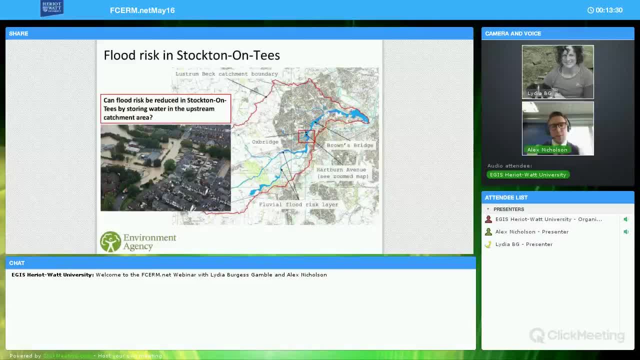 protection up to 1 in 25 year. Phase two of the works is looking at upstream catchment storage to in the form of natural management, to slow, and it's desired that the the natural flood management, or phase two of the works, is able to bring up the standard of protection from those areas that are. 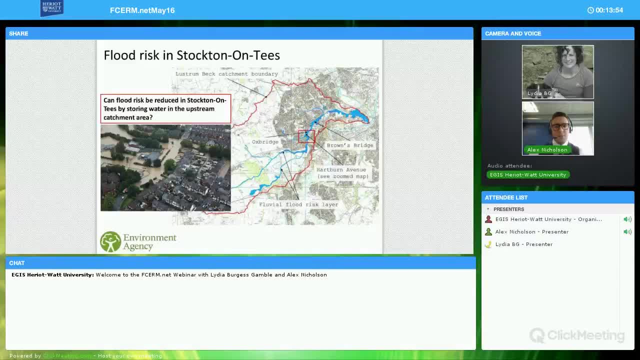 left at 1 in 25 year up to 1 in 5 year, and the areas that are currently at 1 in 75 year to go up to 1 in 100 year or even higher. So how can we begin to consider natural flood management at the scale of 45 square kilometres? 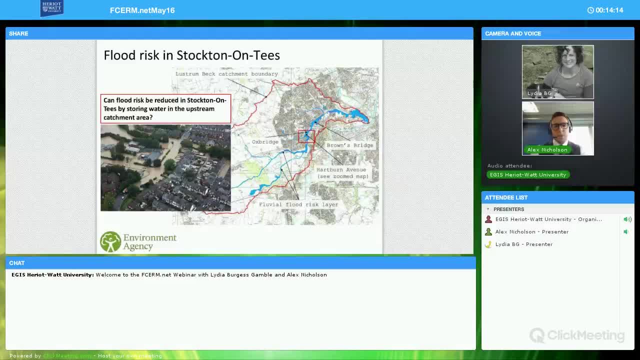 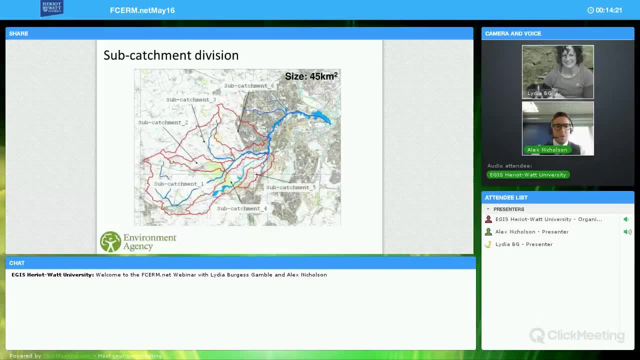 particularly when I've been used to looking at small-scale examples like Belford. Well, firstly, to make it more manageable, I broke up the larger 45 square kilometre catchment into six sub-catchments. This is purely as an idea for me, just to get my head around where it might be feasible. 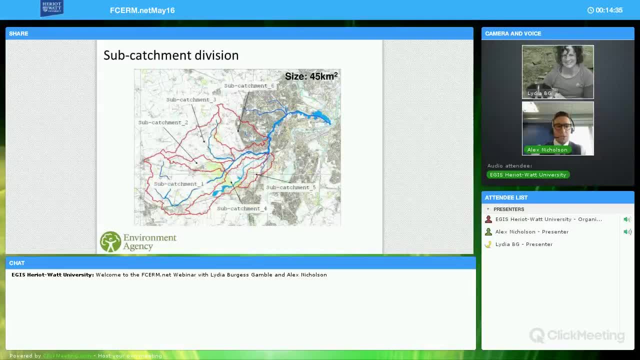 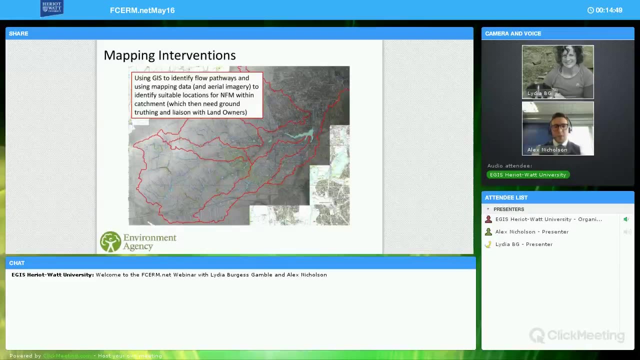 to start situating natural flood management features to slow, store and filter flow. So instead of having one 45 square kilometre catchment, we now have six sub-catchments of somewhere between 5 and 15 square kilometres. I then used hydrology tools in ArcGIS to identify, on the DEM, the LiDAR data, where 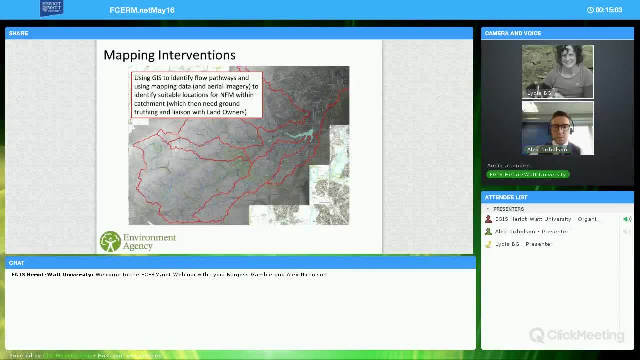 flow pathways would be occurring when rainfall is targeting the site. With the flow pathways in place amongst other layers like fluvial flood risk or surface water flood risk layers, I was able to start identifying where we can start putting natural flood management features in the system. 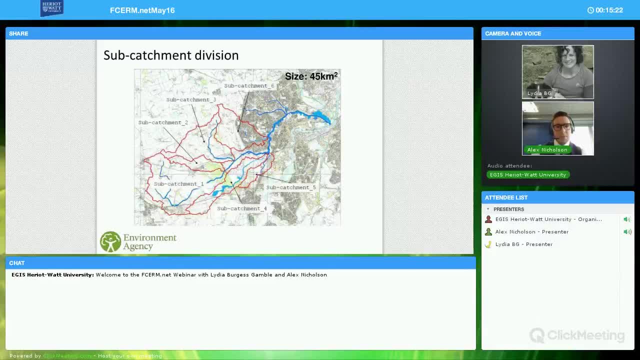 So that's the first step. The second step is the upstream catchment, and so let's just go back to this map of the whole area. We're going to focus in on sub-catchment one just to look at a bit more detail about how. 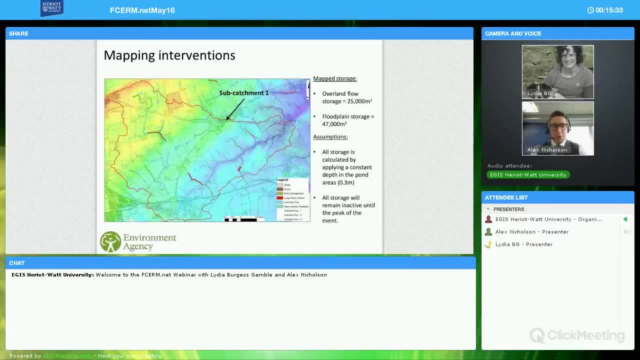 I did that. You might have to squint a bit to look at this, but in the background you can just about make out some runoff pathways which are being picked out by these hydrology tools in ArcGIS. And on to that I've sort of superimposed. 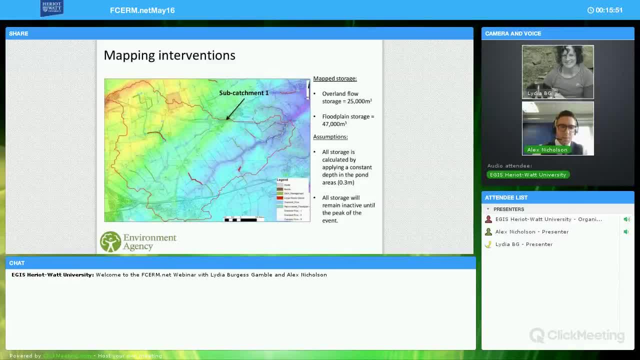 I've superimposed four different types of shapefile, which in this case are a large woody debris, which is the sort of red and black areas. So I've situated those on small streams and ditches which are in the vicinity of an area. 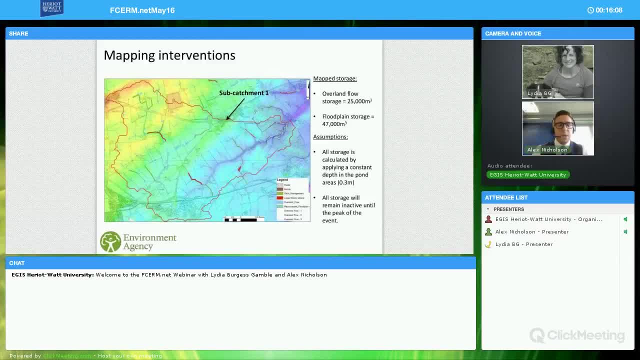 of existing woodland, because that would be where you get the source of wood from, And I've tried to avoid putting them on a catchment area greater than three square kilometres. And this is just based on some research that we did, that we did in Belford, where we basically determined that three square 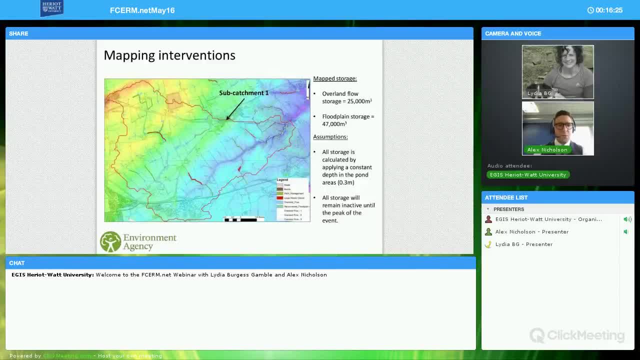 kilometres was kind of this threshold for the forces becoming too great on large woolly debris. Some small green lines you might be able to make out are indicating areas where ditch management might be applicable, and all I'm really referring to there is areas of ditch widening techniques, online storage of 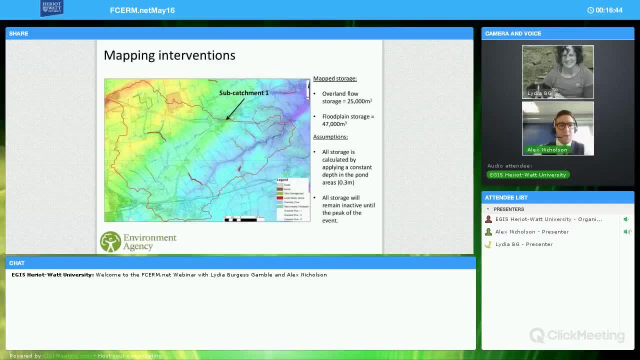 flow to drop out sediment and mass nutrients that might be being washed off farmland during rainfall events. These two components aren't really considered by the modelling, but I've still thought it'd be useful to put them in this opportunity mapping, just because it kind of it's a part of what what we sort of. 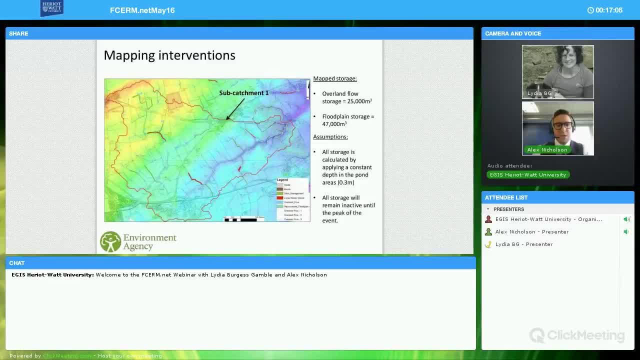 like to term as the multiple benefits of natural flood management. Slowing water in these small ditches and managing sediment and water quality is a big plus, a big tick that we want to try and achieve with NFM. So the other two components that I'm considering here are: 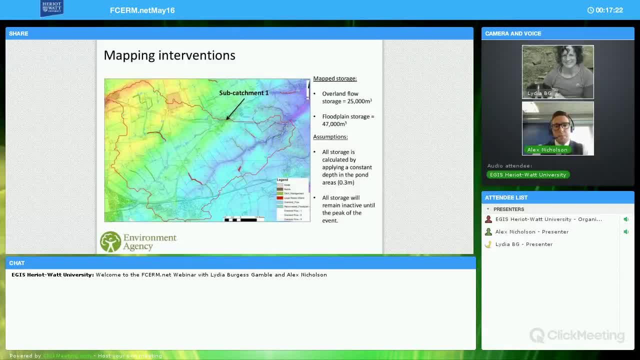 the storage components, the physical storage of water. I'm doing that through the storage of overland flow. so we're intercepting runoff pathways in the land and storing water on farmers fields, perhaps in the corner of fields, and we're looking at flood plain storage. This is, this might be areas of flood. 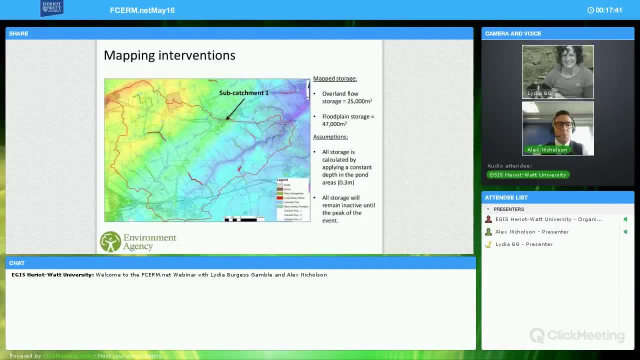 plain that are currently active and we're we're trying to store more water on them by constructing soil buns to increase floodplain depths, Or it might be completely reconnecting areas of disconnected floodplain On the right hand side. I've put a few assumptions, So the storage that I've mapped is drawn as a 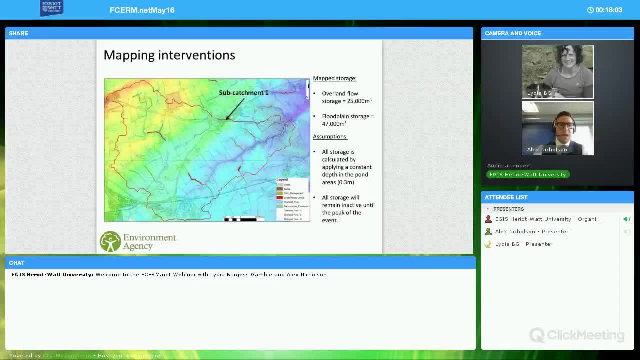 shapefile And then I've assumed a constant depth over the area And that's helped me calculate the amount of storage in each NFM feature. And you can see, in this subcatchment alone we've managed to store somewhere around 70,000 cubic meters of water. Now this is 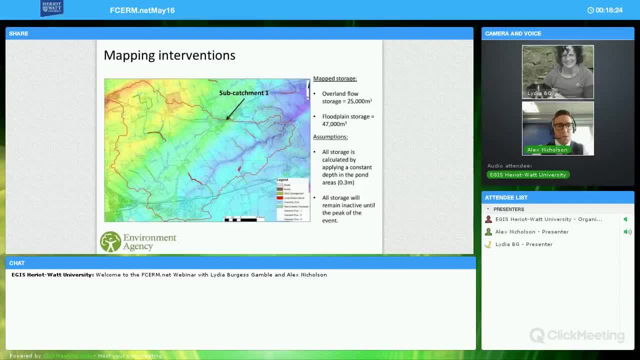 purely up in the air. I'm calling this really no constraints, natural flood management mapping. It's before consulting any landowners And it's basically just using the DEM and a few rules about where you might be able to situate something. I found this field to try and figure out. OK, these are the best opportunities. Let's. 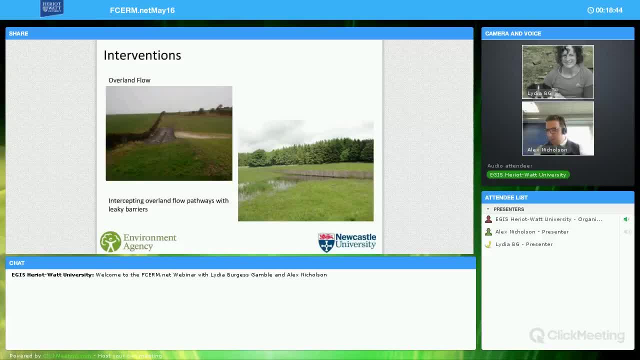 take them forward. Let's go and have a discussion. So just describe what those features might look like. Lydia's already gone over a couple of them, But overland flow features might look like these: examples from Belford: On the left you have a soil bund capturing a. 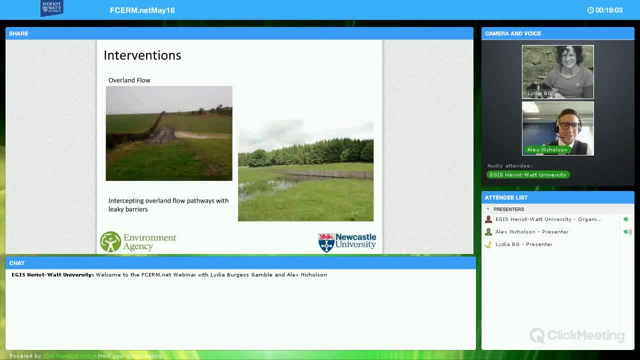 runoff pathway- Sorry, I'm sneezing, OK, Bless you. And the soil bund in this case makes access to the field during wet periods much easier for the farmer, And there's a pipe going all the way through that allows. 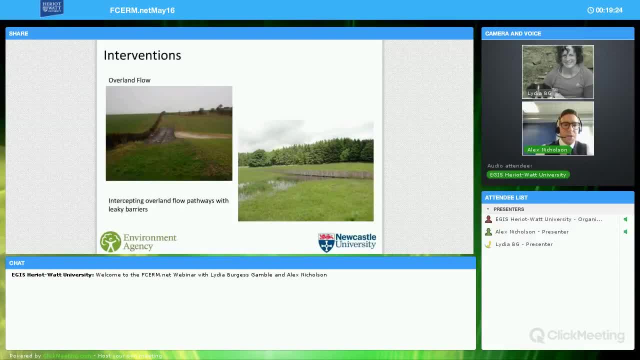 the structure to leak. You'll also notice that it's situated at the edge of the field. So in this arable field case we're not interfering with the sort of function of the field. It's within the buffer zone. On the right-hand side it's an area that's a little bit more. 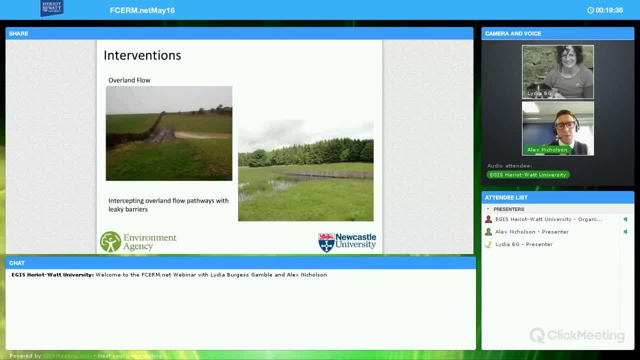 wet. It's a field set for grazing very shallow soils, So this timber barrier was used, The location of which wasn't as important because it was a field always set aside for grazing, So it wasn't pushed right to the edge. It was put in a position where the topography 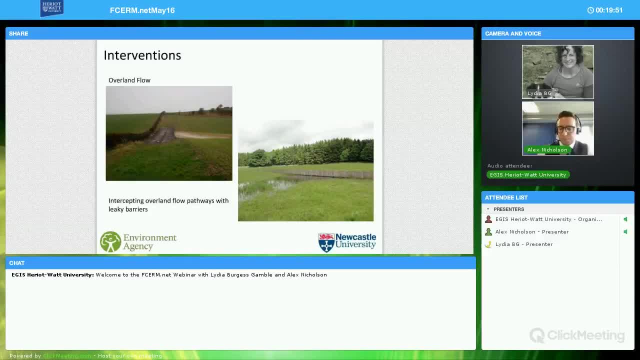 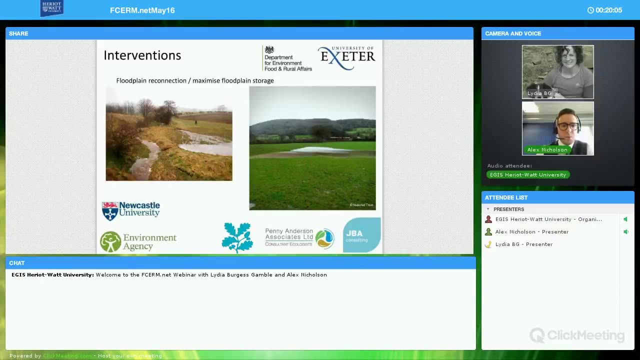 of the field made most sense for it to be. It would store most water. Again, both these features are able to leak and will fill up and empty in a period of less than 12 to 24 hours. Floodplain reconnection and maximizing floodplain storage. There's a couple of examples here. 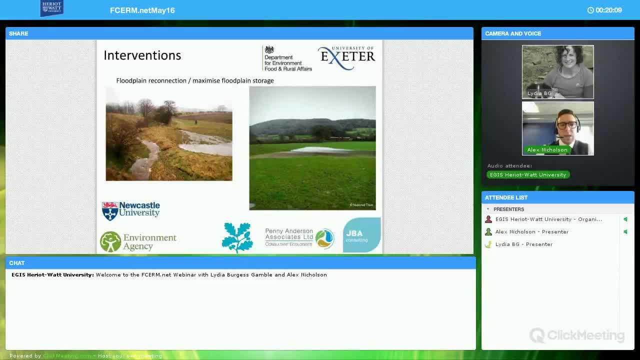 One on the left from Belford of an offline pond. This is basically skimming peak flow, peak river discharge from the burn on the left and pushing it into this relatively small floodplain area on the right which is bunded and is able to store a significant amount. 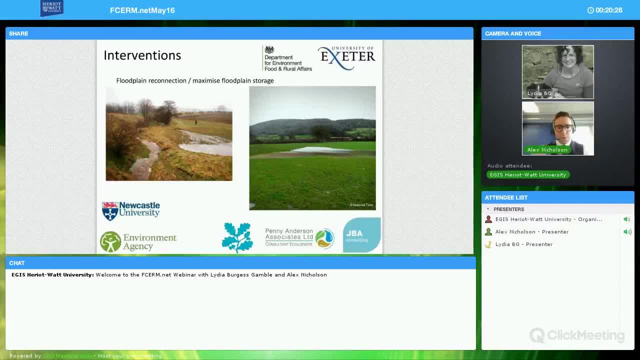 more water than it would have if it didn't have that bund in place On the right-hand side. Lydia has already mentioned a little bit about the flow of the floodplain, So we're going to take a look at the honeycut project. So this is an example that Steve Rose from. 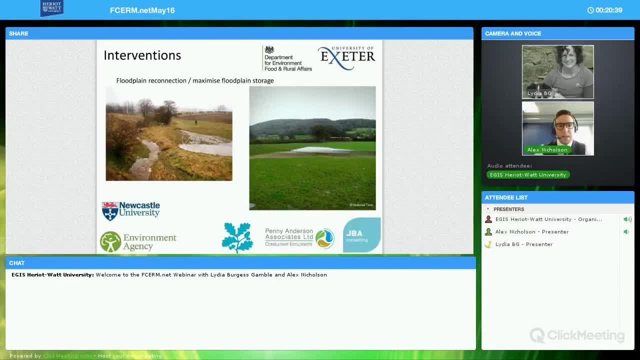 JBA sent and it's basically a shallow, broad-crested bund situated on a large floodplain And there's a number of these And essentially this floodplain was already active, was already able to be active during flood events, And these shallow bunds allow greater depths of storage and 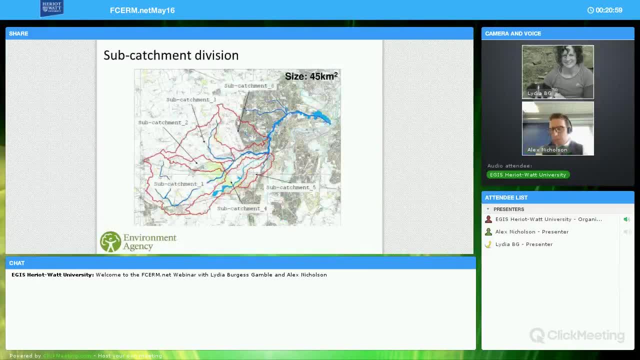 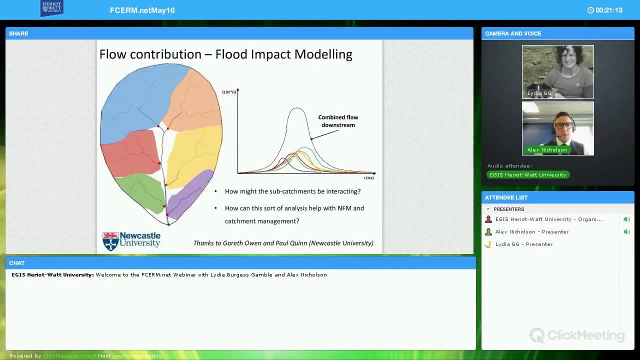 slower propagation of that floodplain flow. Slide 15, Slide 16, Slide 17, Slide 18, Slide 19, Slide 20, Slide 21, Slide 22, Slide 23, Slide 24, Slide 25, Slide 26, Slide 27, Slide 28, Slide 29. 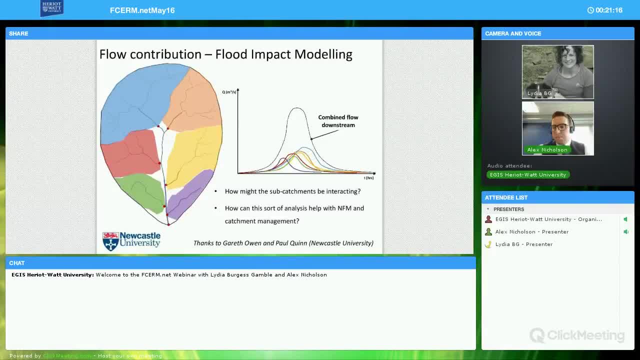 Slide 30, Slide 31, Slide 31, Slide 32, Slide 33, Slide 34, Slide 35, Slide 36, Slide 36, Slide 37, Slide 38, Slide 39, Slide 41, Slide 41, Slide 42, Slide 43, Slide 44. 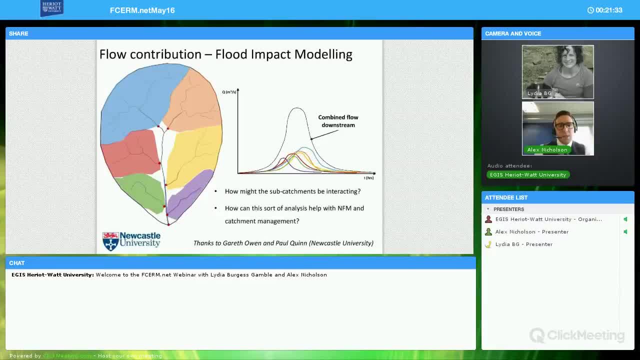 Slide 45, Slide 47, Slide 48, Slide 49, Slide 50, Slide 51, Slide 51, Slide 52, Slide 53, Slide 56, Slide 57, Slide 58, Slide 58, Slide 59, Slide 51, Slide 52, Slide 53. 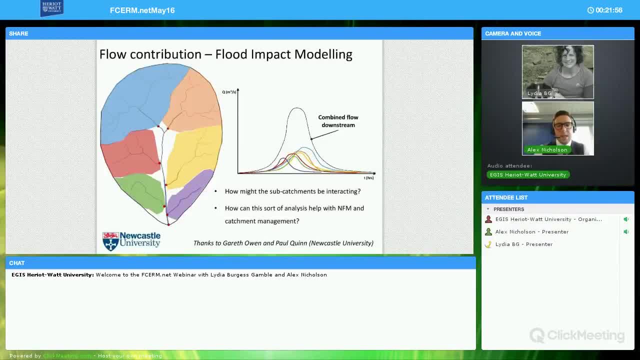 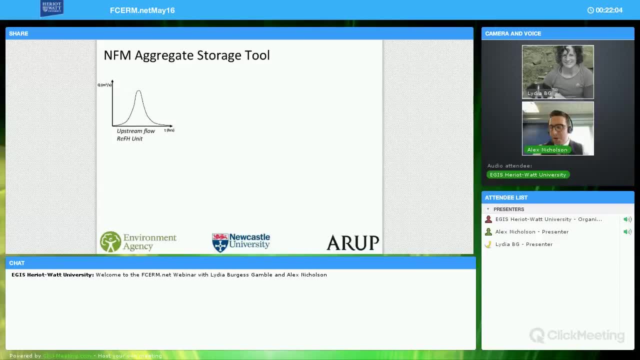 Slide 56, Slide 56, Slide 57, Slide 58, Slide 58, Slide 59, Slide 51, Slide 52, Slide 53, Slide 56, Slide 56, Slide 57, Slide 58, Slide 59, Slide 51, Slide 52, Slide 53. 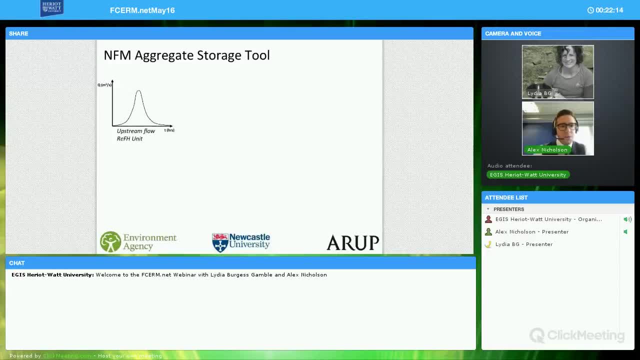 Slide 54, Slide 56, Slide 56, Slide 57, Slide 58, Slide 58, Slide 59, Slide 51, Slide 52, Slide 53, Slide 54, Slide 56, Slide 56, Slide 56, Slide 57, Slide 58, Slide 58. 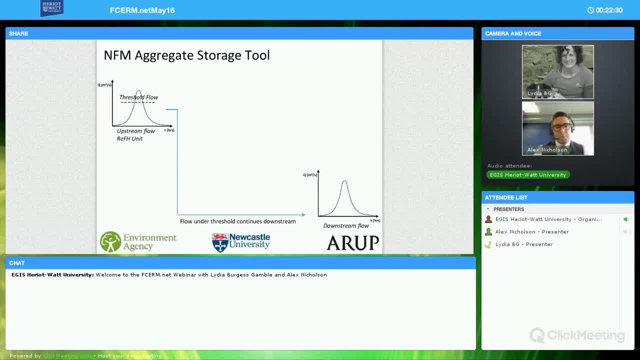 Slide 59, Slide 51, Slide 52, Slide 53, Slide 54, Slide 56, Slide 56, Slide 57, Slide 58, Slide 58, Slide 58, Slide 59, Slide 60, Slide 61, Slide 61, Slide 62, Slide 63. 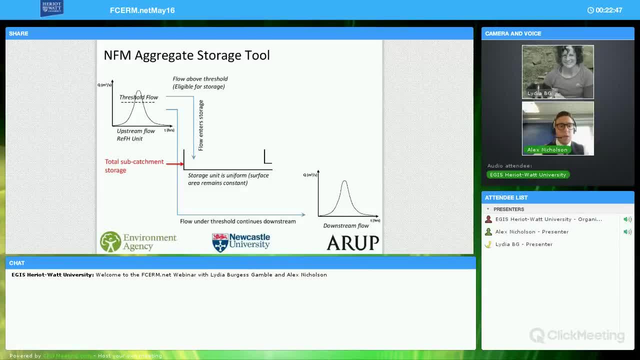 Slide 64, Slide 65, Slide 67, Slide 68, Slide 68, Slide 69, Slide 69, Slide 70, Slide 71, Slide 71, Slide 72, Slide 73, Slide 74, Slide 75, Slide 76, Slide 76, Slide 76. 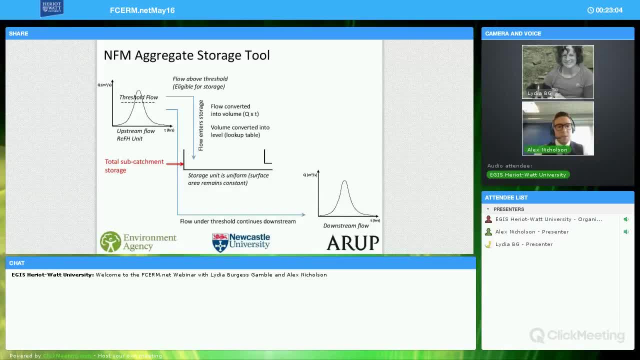 Slide 77, Slide 78, Slide 79, Slide 78, Slide 79, Slide 80, Slide 71, Slide 72, Slide 73, Slide 73, Slide 74, Slide 75, Slide 76, Slide 76, Slide 77, Slide 78, Slide 78. 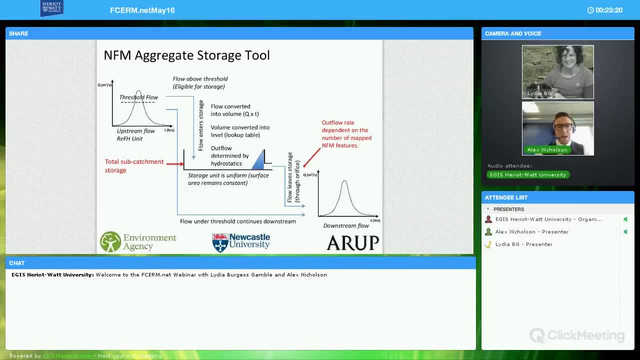 Slide 79, Slide 78, Slide 79, Slide 79, Slide 79, Slide 80, Slide 71, Slide 71, Slide 72, Slide 73, Slide 74, Slide 74, Slide 74, Slide 75, Slide 76, Slide 77, Slide 78. 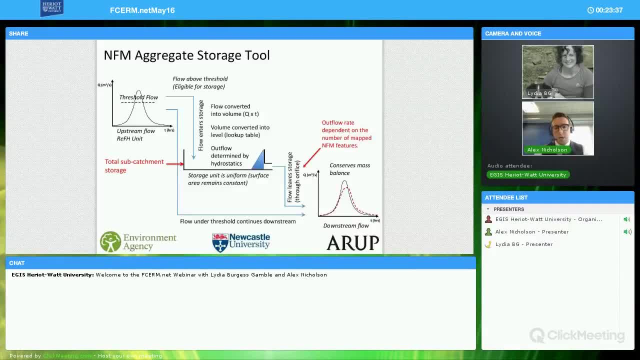 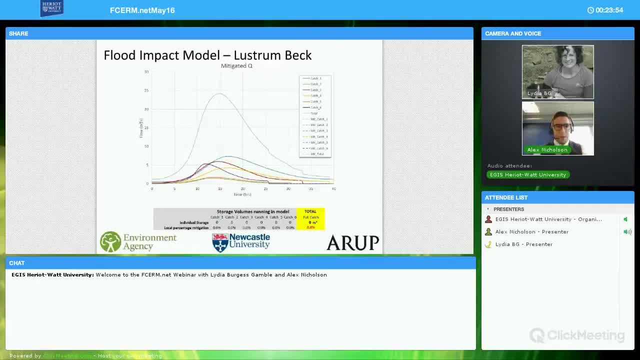 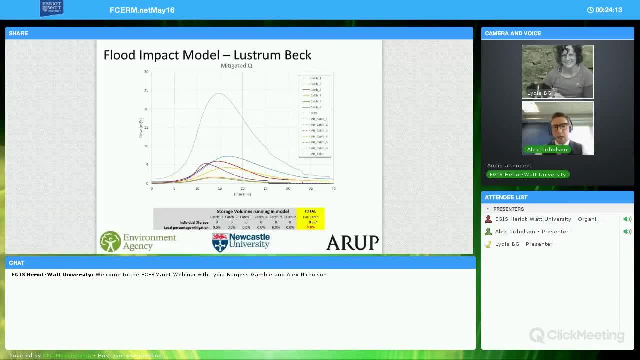 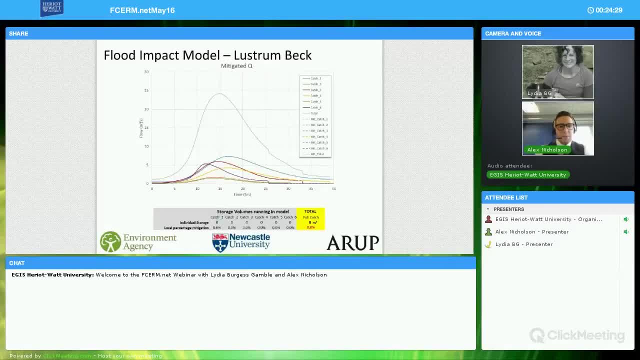 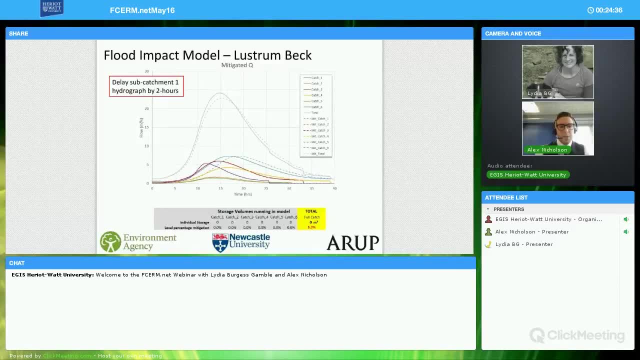 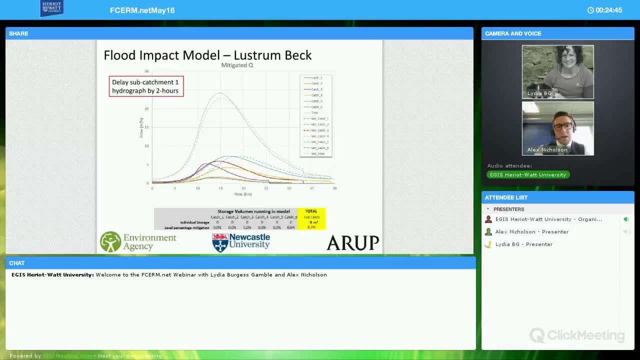 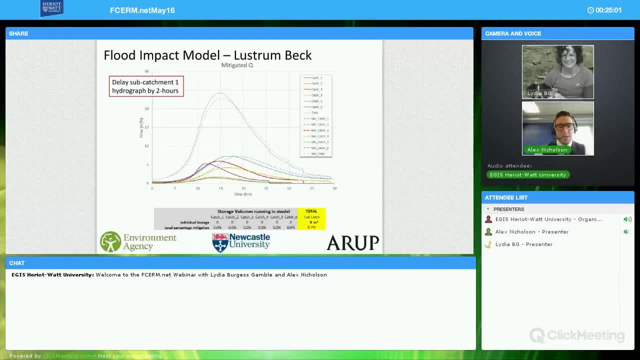 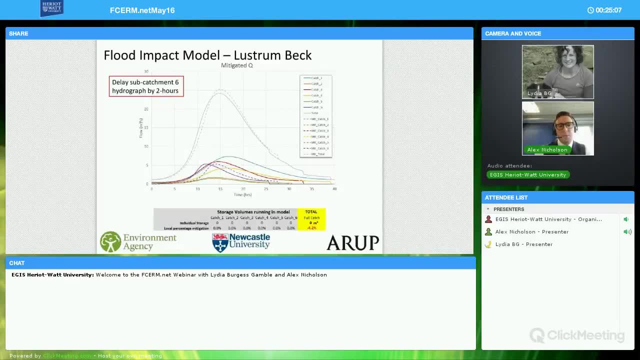 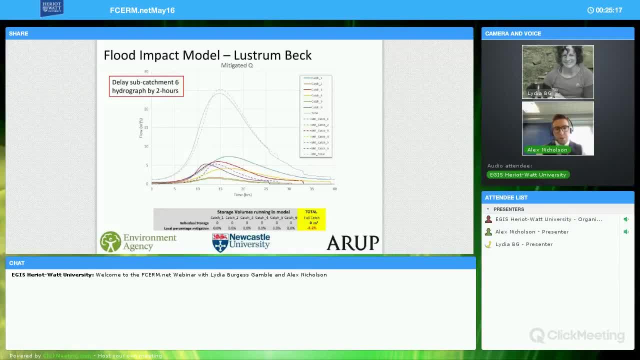 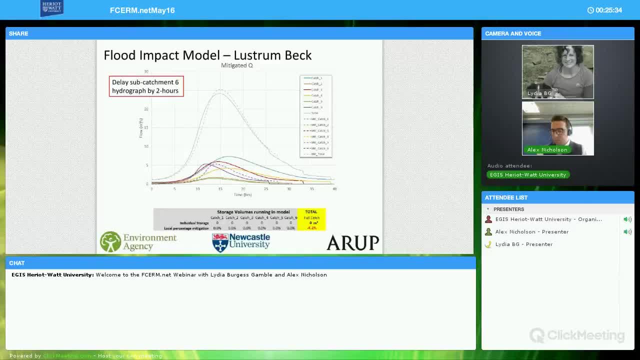 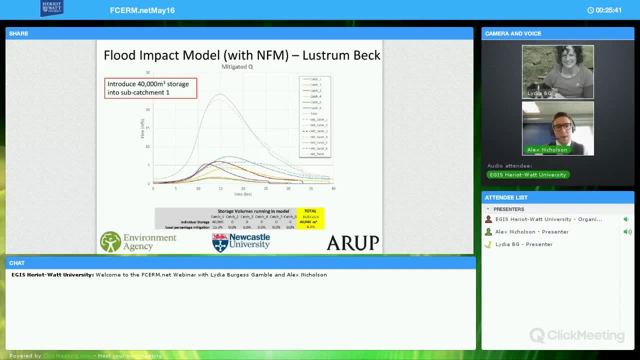 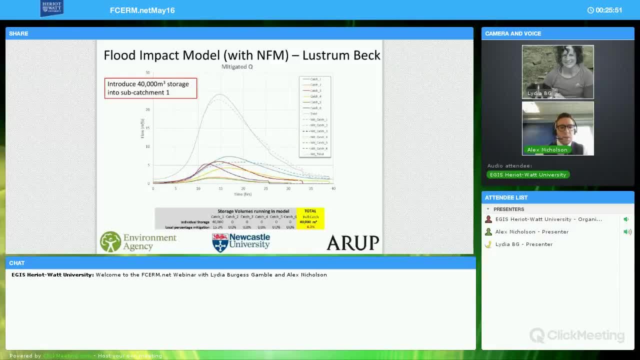 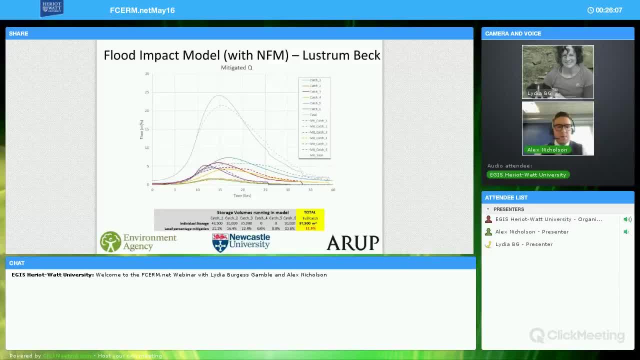 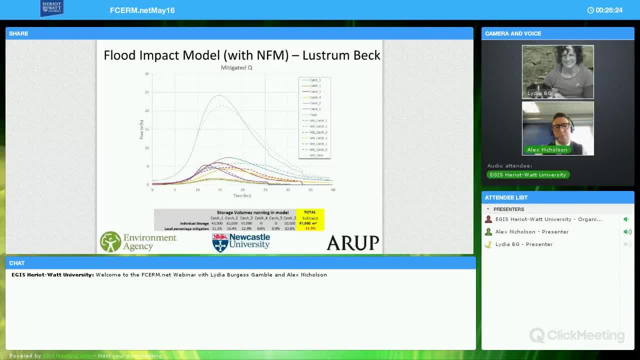 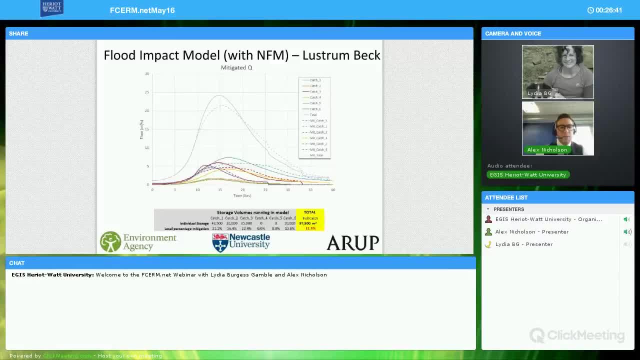 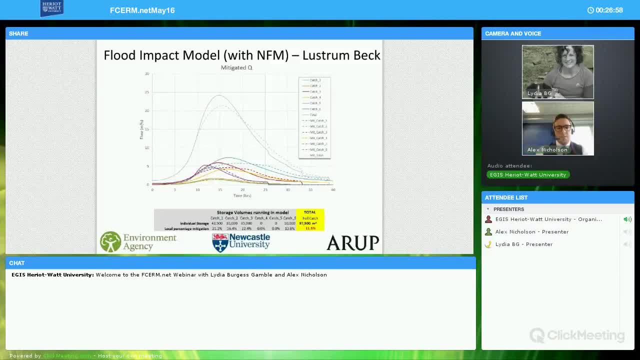 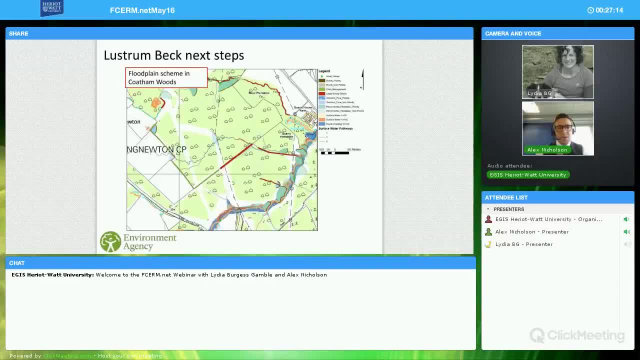 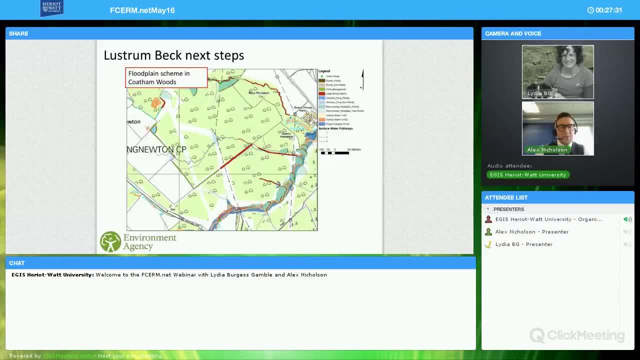 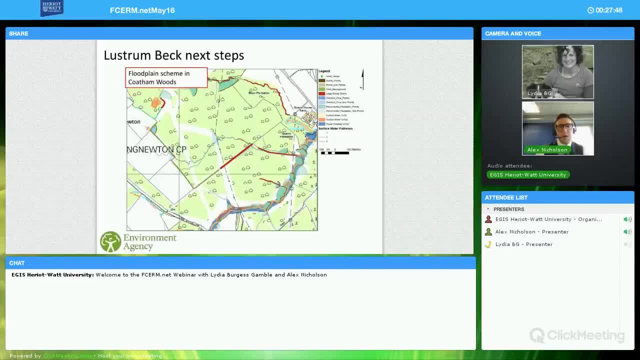 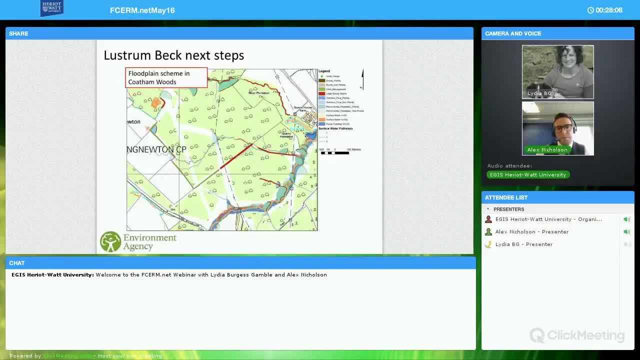 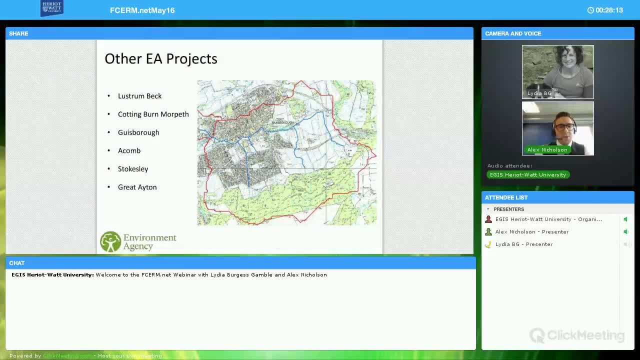 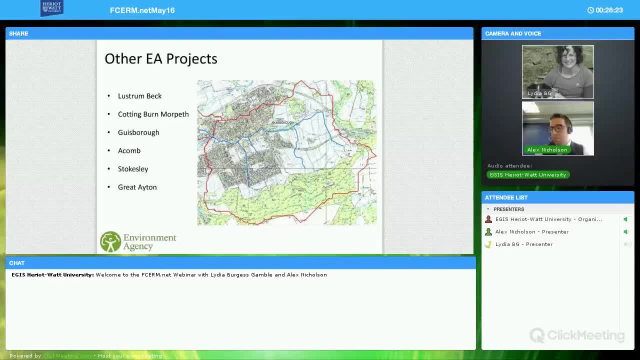 Slide 78. Slide 78: exciting time for natural flood management and hopefully we'll together start making better ways of modelling it and getting it on the ground so that people can be more protected and safer. I'll just pass on to Lydia for some closing points and then we'll take some questions, I think after. 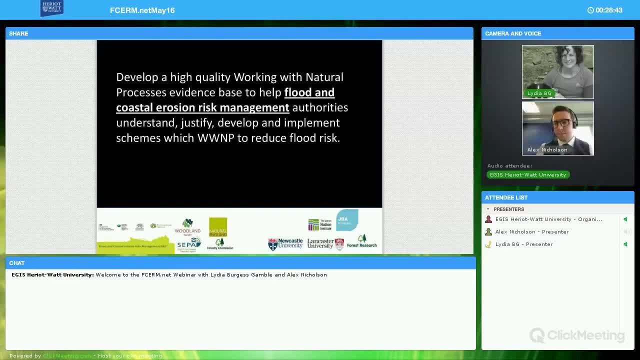 that. Thank you very much, Alex. that was really, really interesting. I think I'll just pick up on what Alex just said, that there's a lot of projects going on in the North East where he works. but what I'm picking up on a daily basis is that there are projects happening all over the UK, everywhere at 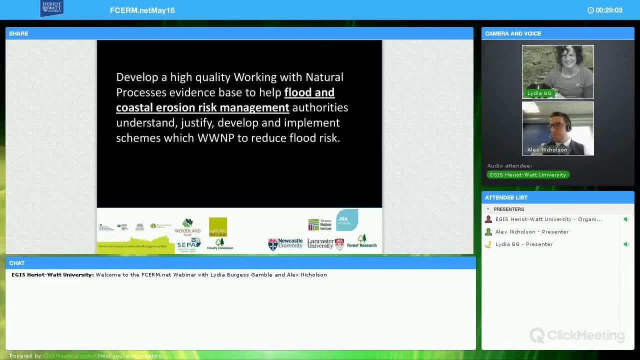 the moment, everyone seems to be starting to do natural flood management projects, so it really is an exciting opportunity, and what I just want to do now, before we hand over to you to write questions in the chat area, is just to talk about some projects that I'm working on at the moment. I'm working on a project that I'm working on in the UK, and I'm working on a project that I'm working on on the project that I'm working on in the UK, and I'm working on a project that I'm working on in the UK. 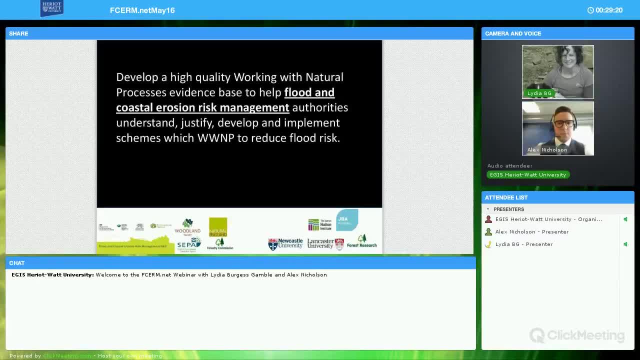 which is all about developing a high-quality evidence base to help support and you guys working flood risk management, to pull together into one place the evidence behind natural flood management, looking at all the suites of different sorts of measures for rivers and the coast, so that we know what to. 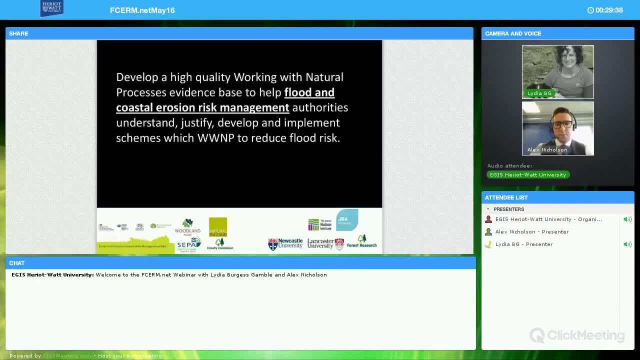 identify what we know and we can identify what we still don't know so that we can be more confident when we're trying to develop the case for natural flood management within catchments- and this is a project that I'm managing for the Environment Agency, but it's a big partnership project with contributions. 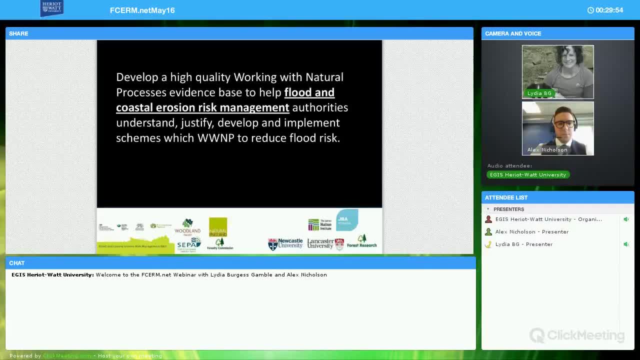 from SEPA and the Woodland Trust and our contractors are our JBA in the consortium with Forest Research and Newcastle Uni, Lancaster Uni and the James Hutton Institute. so this is a 18-month project which started in February and it's got various compartments to it, but it's all about. 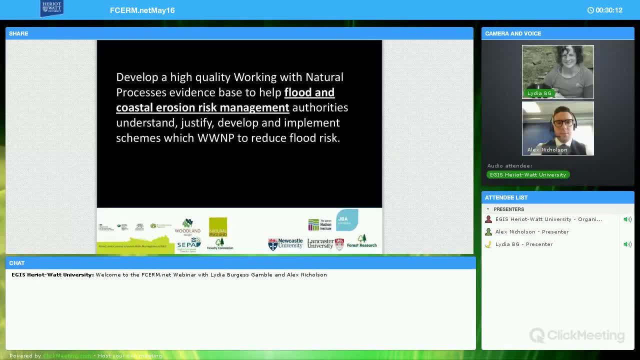 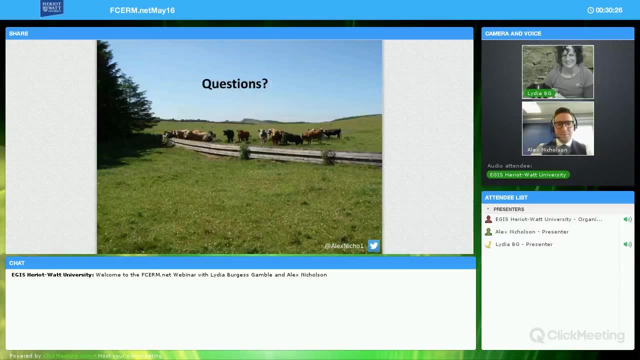 pulling together that evidence into one place so that natural flood management can be considered alongside more traditional forms of engineering. so thank you ever so much for your time in your lunch giving your lunch break to Alex and I. but if you'd now like to let us know if 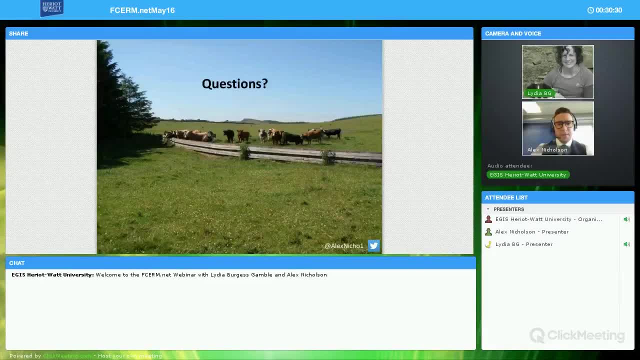 you've got any questions, I believe if you write them in the chat area, what I'll do is I'll read them out and then either Alex or myself will answer them. so fire away. if you've got any questions or if you feel like you need some more information, please feel free to reach out to Alex or myself and we'll answer them. so fire away if you've got any questions or if you feel like you need. 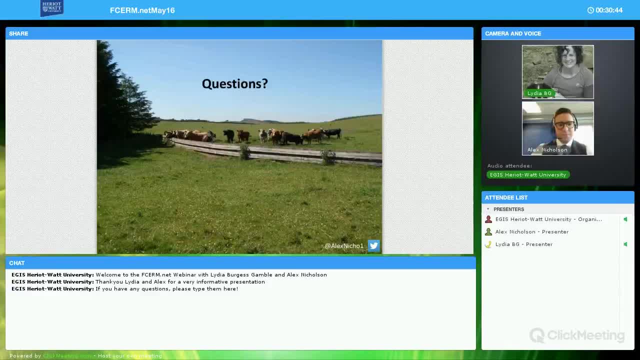 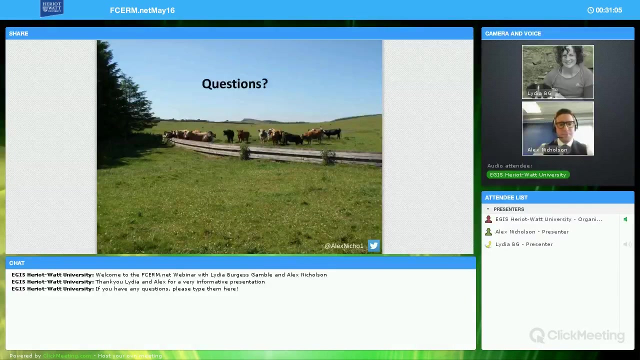 some more information. please feel free to reach out to Alex or myself and we'll answer them, so fire away. if you've got any questions or if you need talk to us offline, then please contact us. so we just- yeah, I think you just typed them into the chat area. sure, there must be some questions, but whilst 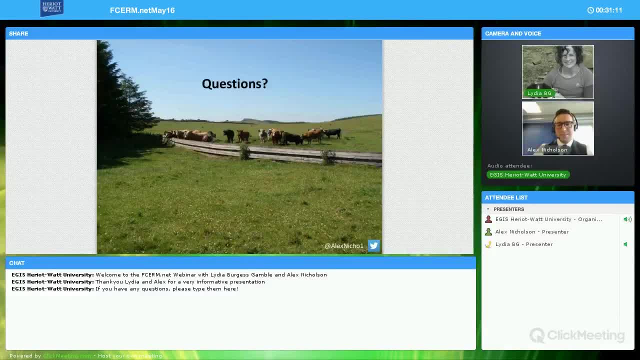 you're all thinking of questions what what we will do is. we're a After this event. I believe Harriet Watt will send around a recording of our webinar so you have that for posterity, But we will also add a link to where you can get access to the reports. 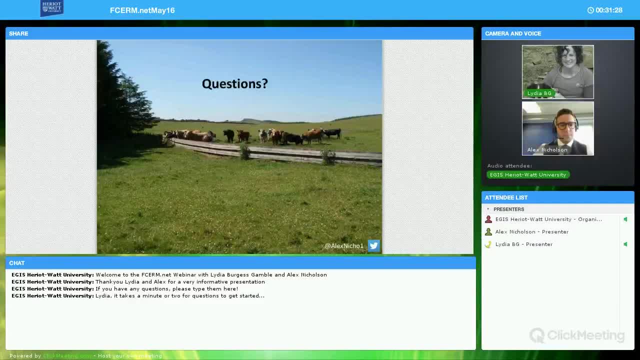 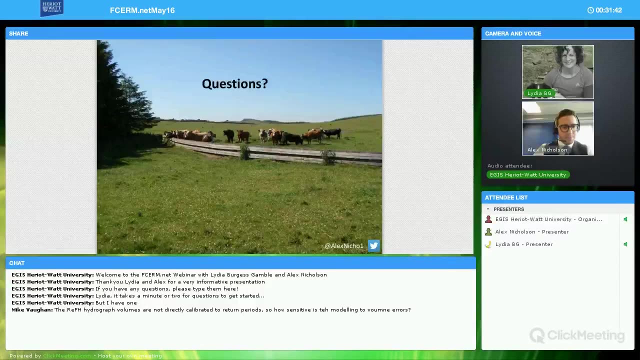 that I've been talking about and provide you with our email addresses if you want to speak to us directly. I think we've got some questions starting to come through, So if you want to hold the line, One from Mike Vaughan. The question is: the REFH hydrograph volumes are not directly calibrated to term periods. 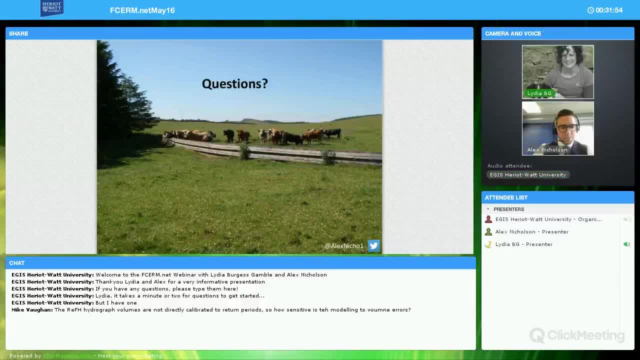 So how sensitive is your modelling to volume errors? I think that's one for you, Alex. Yeah, I'll try and answer that one. Well, thanks, Mike. It is a very simple representation Of a situation here. What we did was we applied. we made sure that the critical storm duration 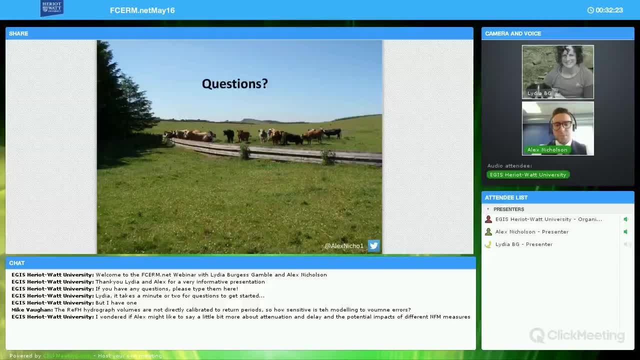 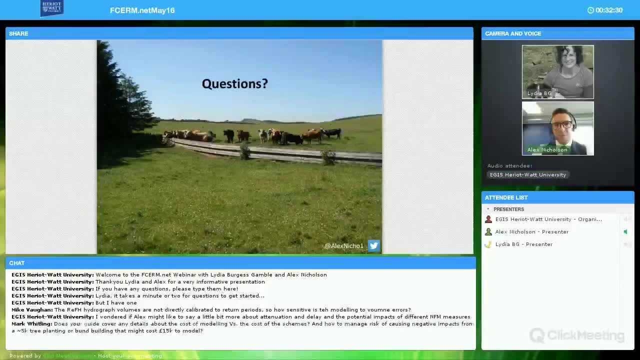 for the REFH hydrographs was adequate for a heat being the worst flood condition downstream. But absolutely these are. there is a huge scope for error in this analysis. It's essentially looking at Turning a baseline case, which is a hydrograph, into a design case, which is a hydrograph plus. 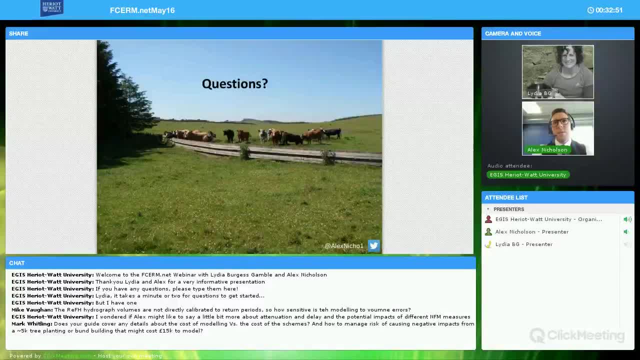 So if there are volume errors in the in the REFH hydrograph, those would be represented in the base, both the baseline and the design case. I hope that answers the question. But yeah, again, it is very simple representation of what's going on. 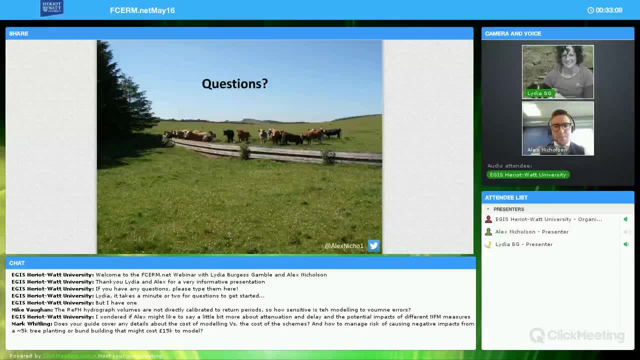 OK, and we've got one from what here Which said one of Alex would might like to say a bit more about attenuation and delay and the potential impacts of different MFN measures. OK so, OK, yeah, so the difference between delay and attenuation. 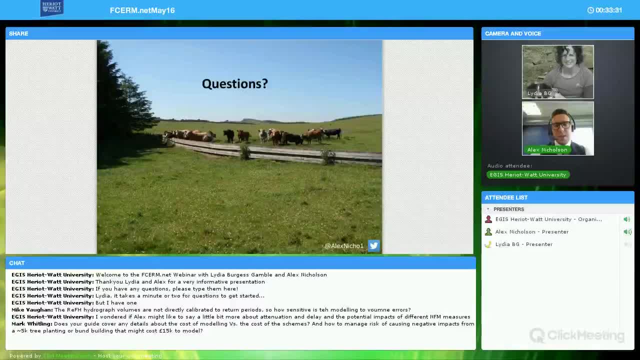 Well, what we're sort of getting out there is that I mean, attenuation and delay are the same thing, but The MFN is just total storage. We're not. we're not saying that, that we are simply storing and subtracting an area of or amount of water from the hydrograph. 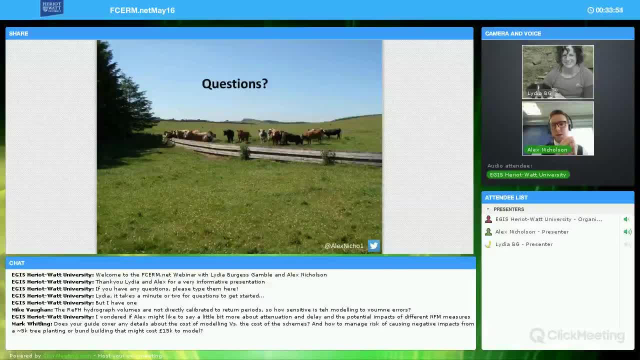 We're. we're taking that water from the graph and delaying its approach through the system. So the same amount of water is coming out downstream. It's just coming out in a different sort of pattern And some of the We were getting from Belford- although it was very small because we were looking at individual features- we were able to measure a delay effect from pond to pond. 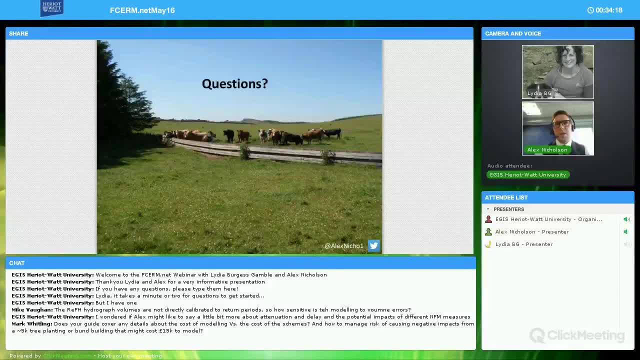 But what we weren't able to physically measure was the, the combined effect of all that, all that storage in the catchment, So what? what we ended up doing was creating this tool, unimaginatively called the pond tool, that emulated the effect of one pond. 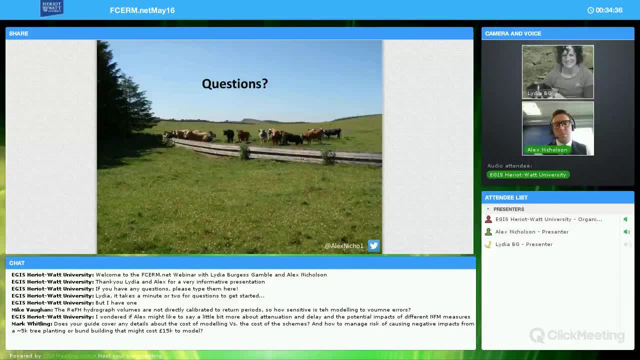 And like, like a series of Strung together. So we were able to say, well, this is what we've measured from one And this is what we think would happen with having 30 features of this type in a row. OK, I think got a question for me from Mark Whitling, which is the guy's covered details about the cost of modeling, the cost of the scheme and how to manage the risk of causing negative impacts from the 5K tree planting or bunds. 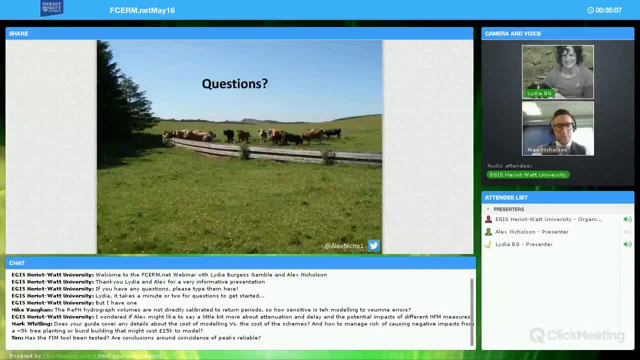 That might cost 15 K to model. So what it does talk about in our report is is about the proportionality of of of modeling. So there are. there's an example from, I think, a shroud example, where I've been doing detailed modeling. 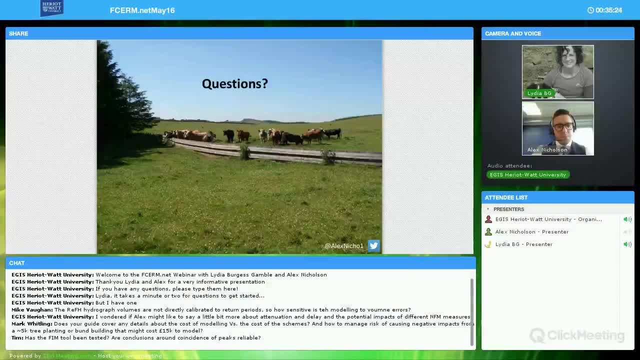 What they do was a really rigorous desk based study and catchment walk over, which helped identify the best places for the scheme. So it talks about not modeling not always being the answer, not always being necessary. it's got to be. you've got to think about it. on a 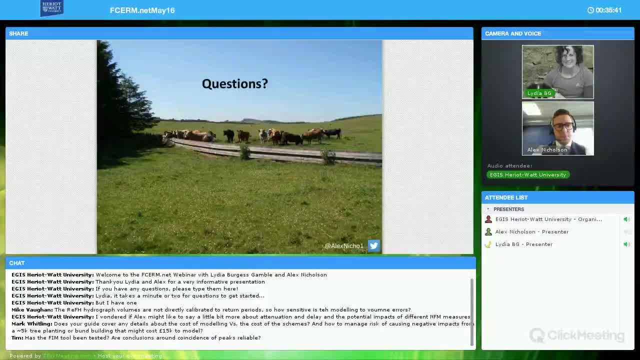 case-by-case basis, because if you're doing a really small scheme, spending three times as much on the scale on modeling as you are on the scheme wouldn't make a huge amount of sense. so it's thinking about proportionality and the risk downstream. so we've got a question from Tim here and which says: 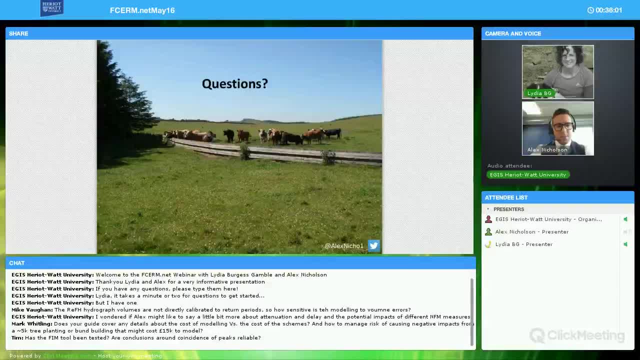 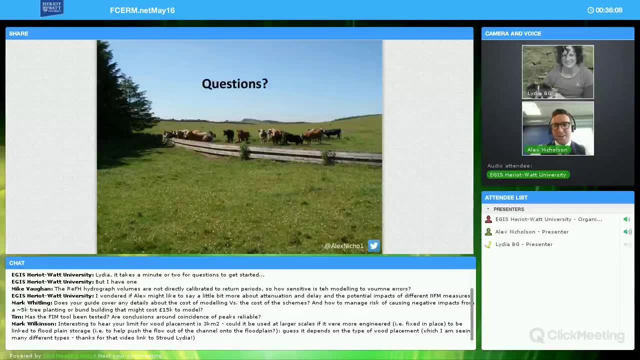 has the FIM tool been tested? our conclusions around coincidence of peaks reliable? I think that's one for you, Alex, there's a good question, I mean. well, what I've managed to do is take the, the FIM tool, and represent it in a in a more. 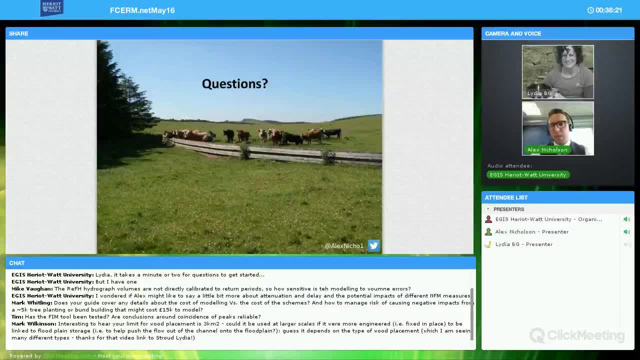 standard Isis format, where, where routing is considered as well. saying that the, as you say, the FIM tool is a more standard Isis format, where, where routing is considered as well, saying that the, as you say, the coincidence of peaks is sort of in the way that I presented it just then it's. 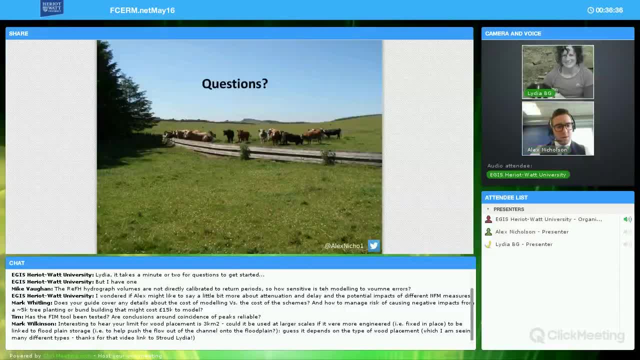 sort of basis based on having a oh, have I back? yeah, you, we missed the start of that answer. you might, yeah, you might, want to start again. sorry, okay, well, I. it was a really great answer. it's a shame you missed. no, what I've managed to do is: 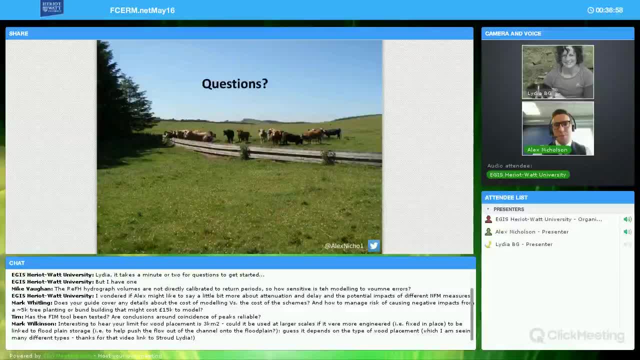 I've turned the, the, the FIM tool, into a more robust representation within Isis to look at peaks coming from different areas of a larger catchment and and therefore we get the routing effect, the sort of, through the system. but what it all is based upon is: is this sort of blanket rainfall occurring over the entire? 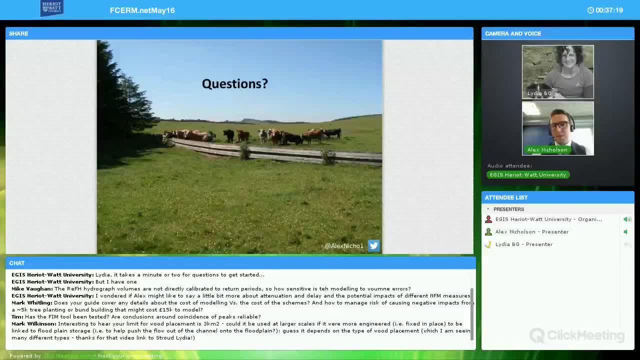 catchment area and those those hydrographs are being generated based on the sort of critical storm duration at the point of interest. so there could be certain scenarios where, for example, rainfall tracking might go one way over a catchment or another way and therefore some assumptions that we have might be more different, with a different pattern of 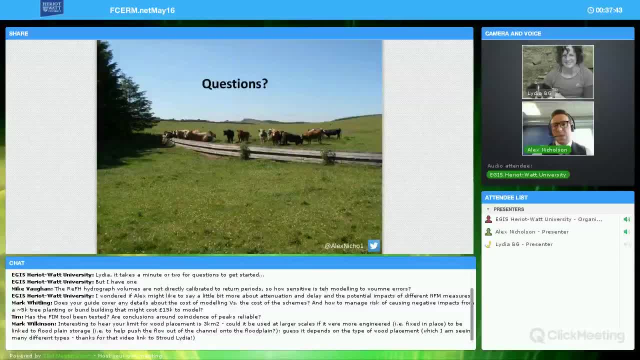 hydrographs and a different timing of hydrographs, and so that's something that definitely needs testing options, test and went before something is really looked into. on the small catchment scale it's not so much a problem, but yeah, as you say, the the coincidence of peak timings does a. 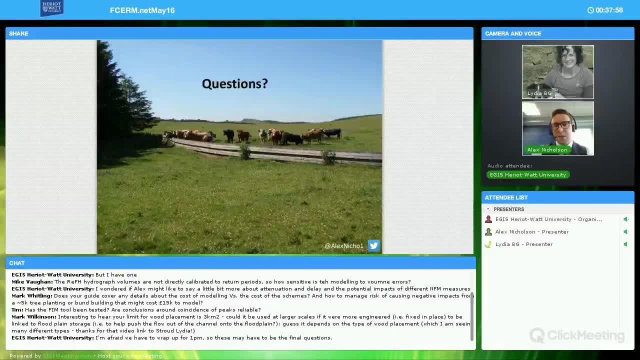 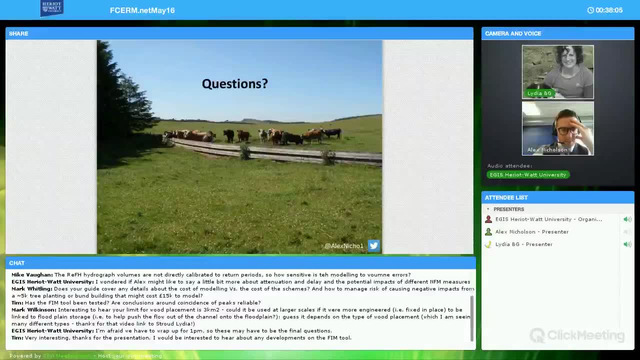 at the large catchment scale. so that's something we need to look in a bit more detail and do some sensitivity analysis on that. We've probably only got time for one more question. We've got one from Mark Wilkinson here which says interesting to hear about: your limit for wood placement is 3km2.. Could 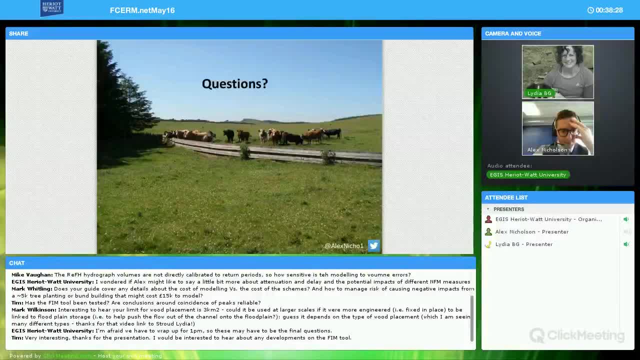 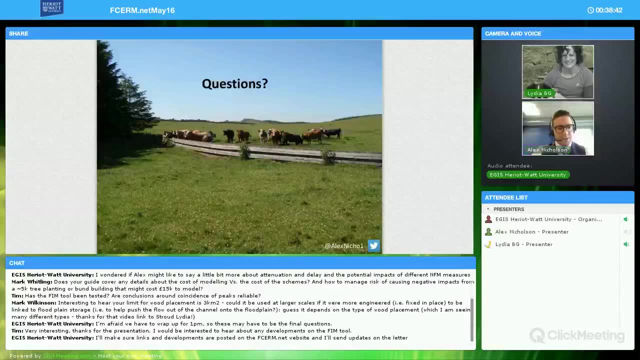 it be used at larger scales if it were more engineered, ie fixed in place to be linked to floodplain storage to help push the flow out of the channel onto the floodplain. So that's probably the last question we can take, so I'll just let Alex respond to that before. 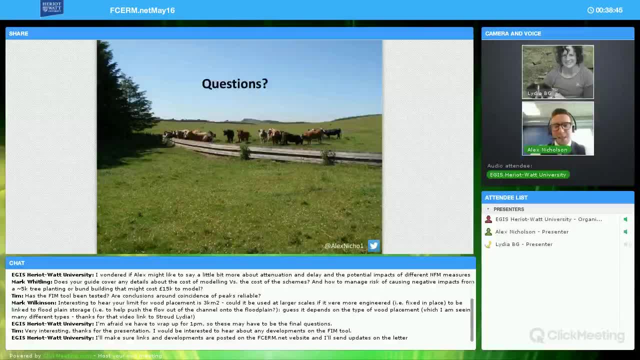 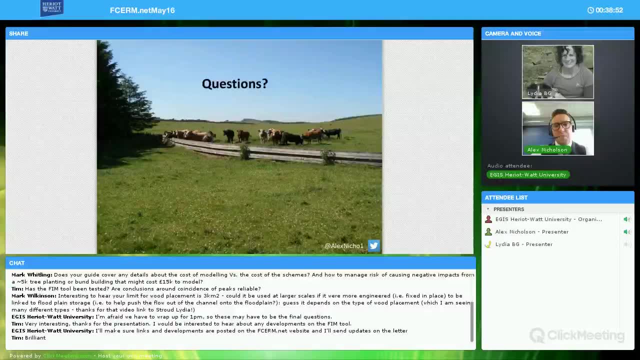 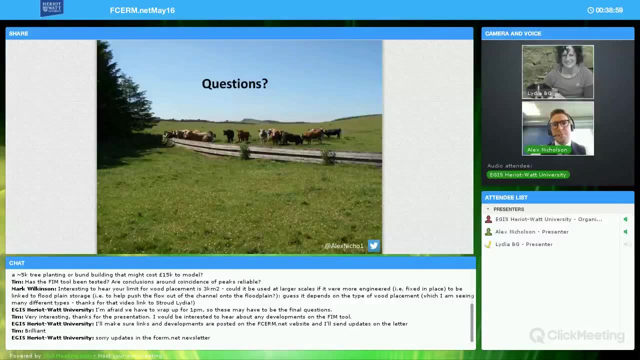 we wrap up. Okay, thanks, Mark. Yeah, I am talking particularly in this case about large woolly debris in the form of naturalised woolly debris, so interlocked large tree trunks. but what we want to make sure is that they're not all the same, probably not rigidly fixed, So 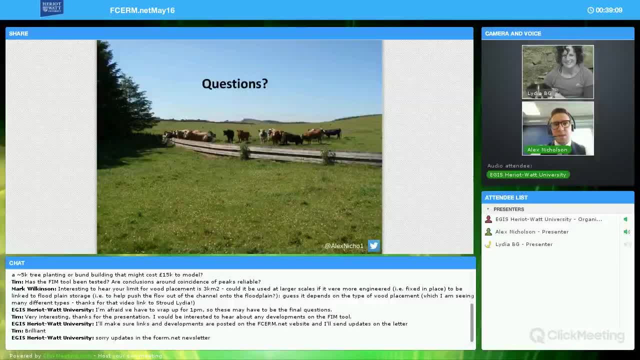 I think, yeah, if it's more engineered, if it's more robust, you could do it on different scales. I think it's more of a sort of nervous thing that, especially when talking about areas close to urban areas and culverts sort of thing, we don't want to make more of an 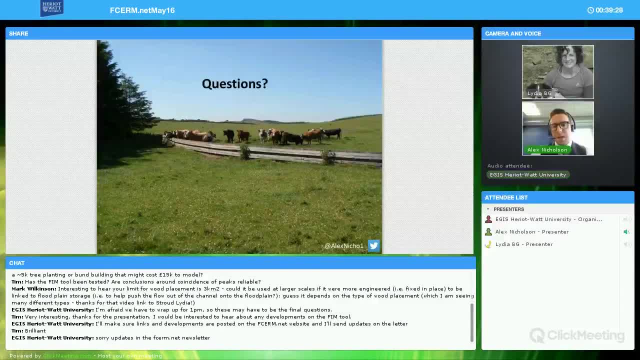 issue than we already have. But yeah, if there's any issues, we'll be happy to answer them. Thank you, Thank you. So if they're engineered and it can be insured through modelling and by design that something won't move based on the design flows that are going through it, then why not go a bit? 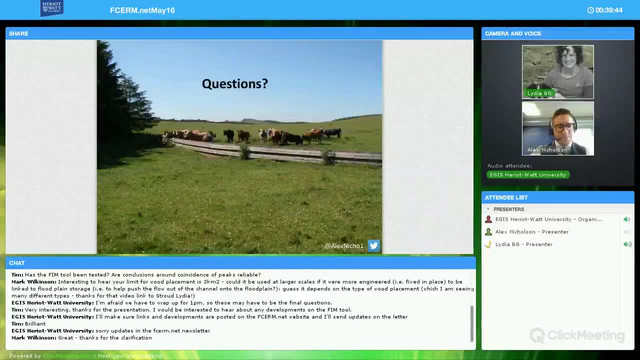 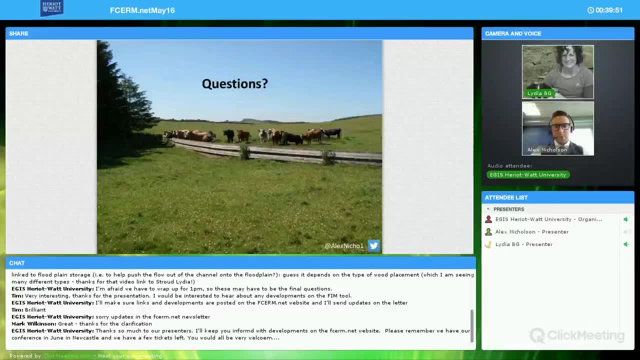 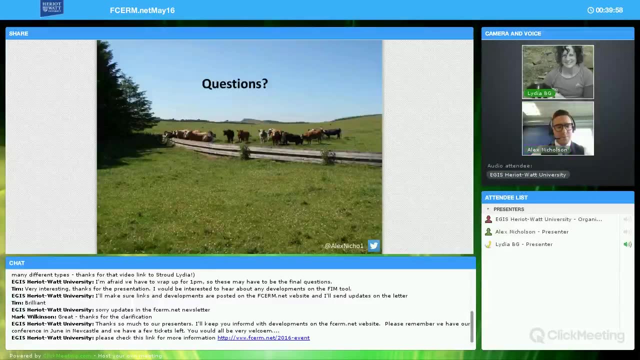 further downstream, Absolutely Okay. Well, thanks everyone for your really great questions. We're going to have to wrap up here. Catherine's going to send around the details from this presentation and presentations via FCR on their web page and via their newsletter. 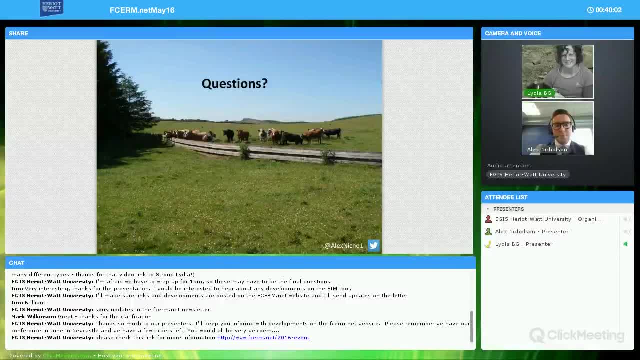 So you better get access to this so you can listen to it in your spare time or share with your colleagues. So thank you very much for spending your lunchtime with us. That's been great. Thanks then, Bye, Thank you, Bye, Thank you. Bye.